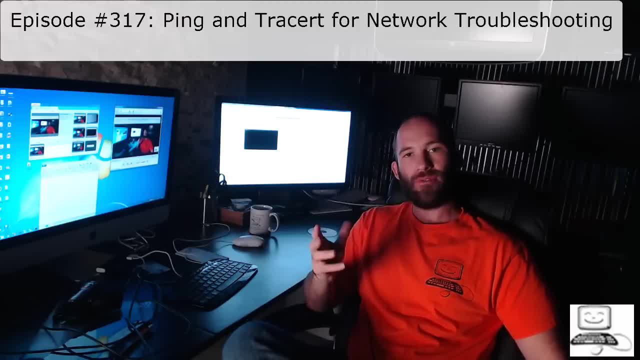 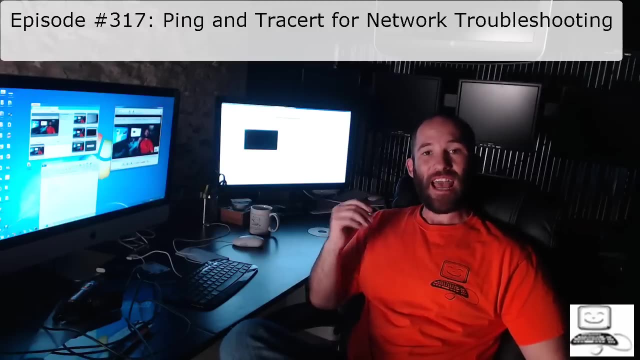 These are just really really great simple tools to use and they will make your life a lot easier. So both Ping and Trace Route are basic DOS commands. they're basic DOS programs and basically what they allow you to do is be able to go out on the network and communicate and see if other computers or network devices are there. 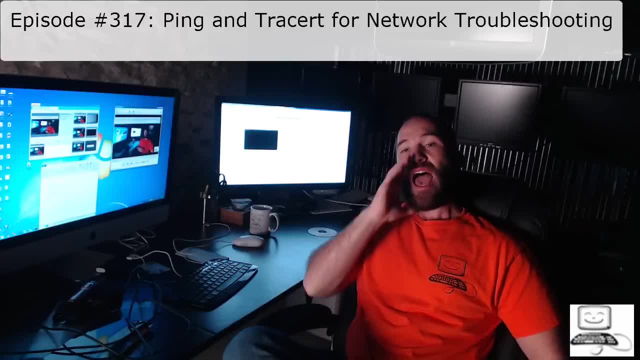 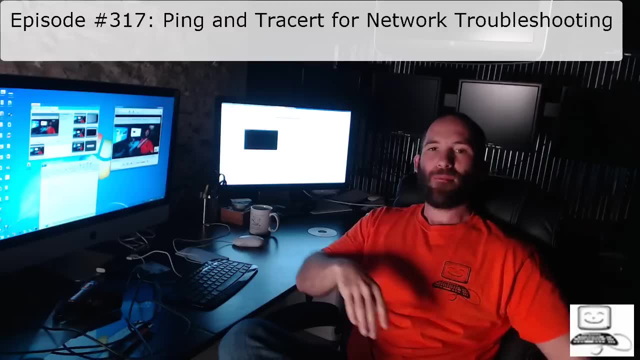 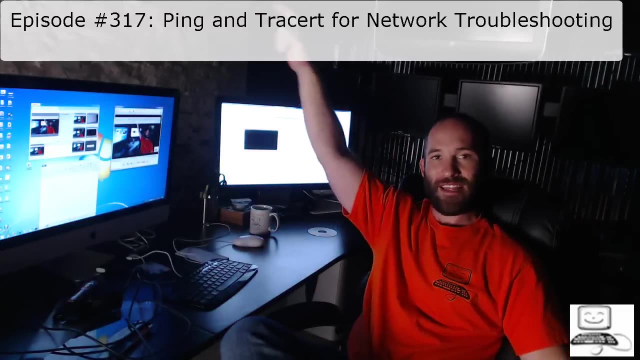 Essentially the idea with Ping is saying, hey, computer number 5, are you there? And computer number 5 will say, yeah, man, I'm here. So imagine if you were like in a cube farm. So you're sitting in your little cube and you want to see if your friend is over in his cube, like five cubes down. 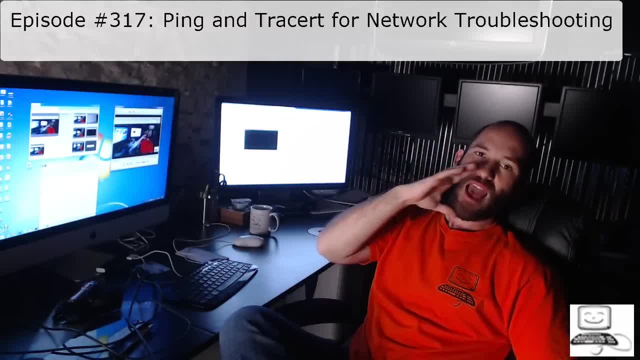 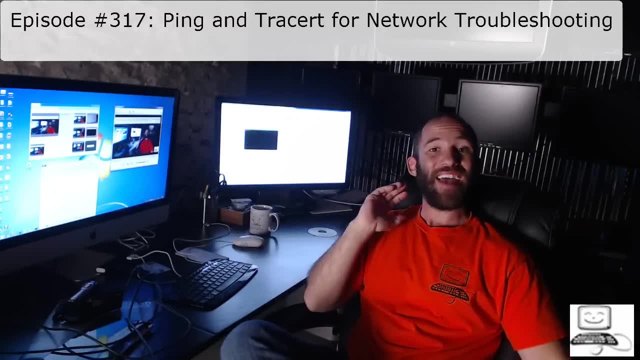 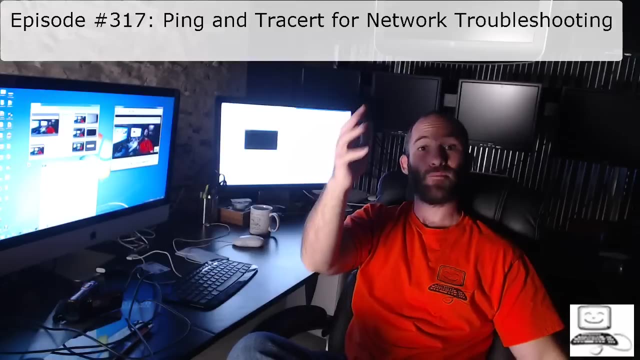 You might say, hey, Bob, are you there? And if he says yeah, I'm here, then you know he's there. If you don't get a response, then you know he's not there And that is all it is. That's about all the communication that happens is all you do is see if the computer or the device is present and is functioning or not. 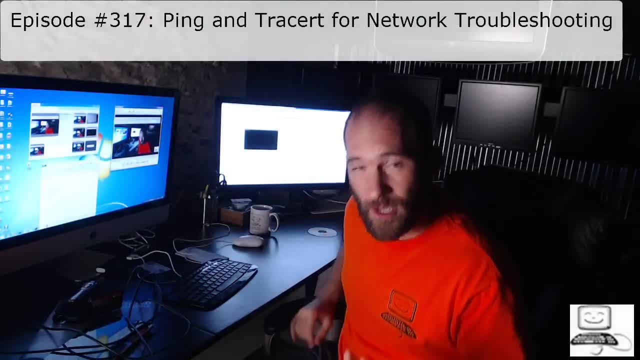 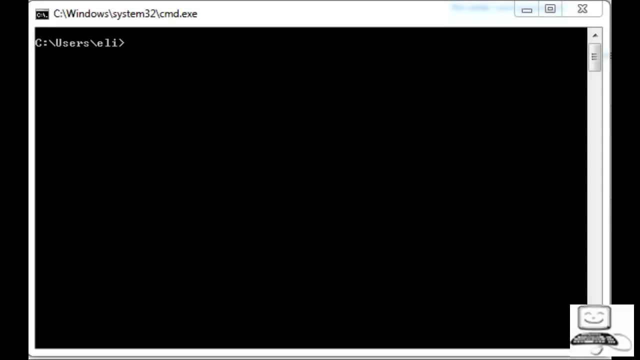 So, basically to show you how how the Ping command works before we go into the troubleshooting methodology, I do just want to go to a command prompt screen. So this is a basic command prompt screen. Whether you're using Windows 7,, Windows Vista or Windows 95,, you will go to this command prompt screen. 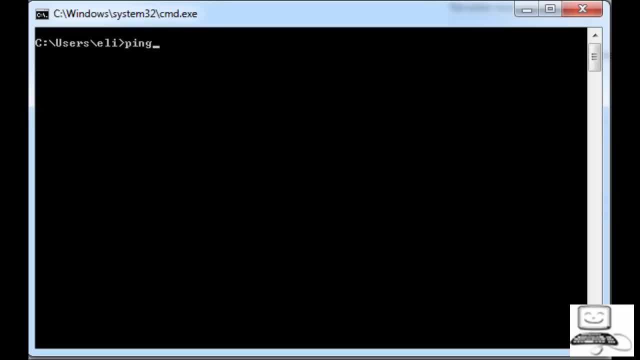 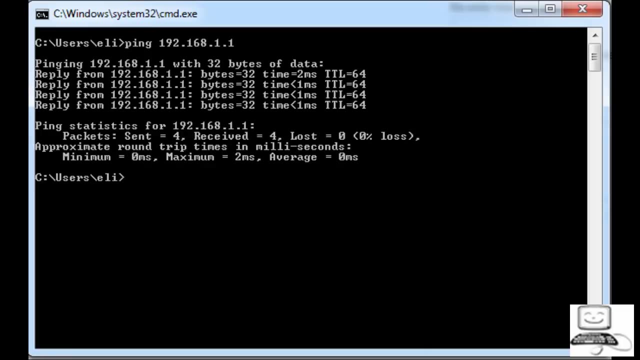 And then you just Ping whatever device you want to see if it exists. So I'll do a Ping 192.168.1.1. And this is my router and I will see if it is there. So it Pings 192.168.1.1, and we can see that it says reply from 192.168.1.1,. bytes equals 32,. time equals two, time delayed equals four TTL. 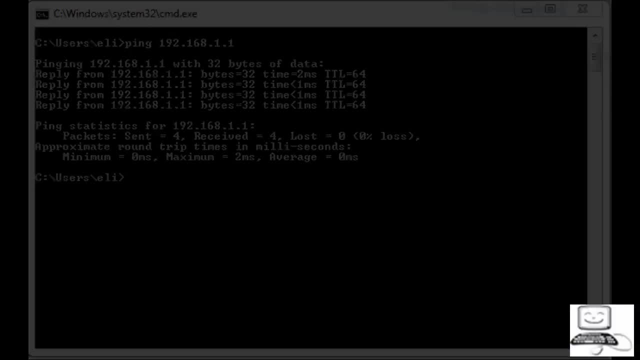 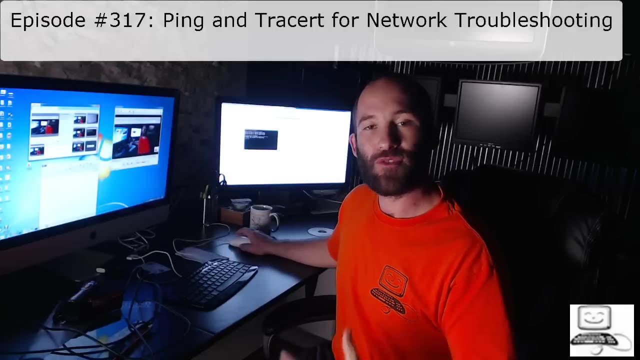 So we know that that IP address is active and it is responding. We don't know what it is. I know it's the router, because I in fact know it's the router. We don't know what it is. do know it is up and running. so if we go here and then let's say we ping. 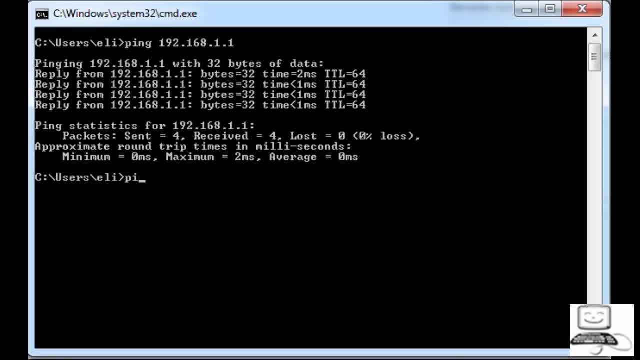 something that I know is not active. so I do ping 192.168.1.222, then we will see that it tries to ping and it's trying, but then we see reply from 192.168.1.3 that the host is unreachable, so that we will. 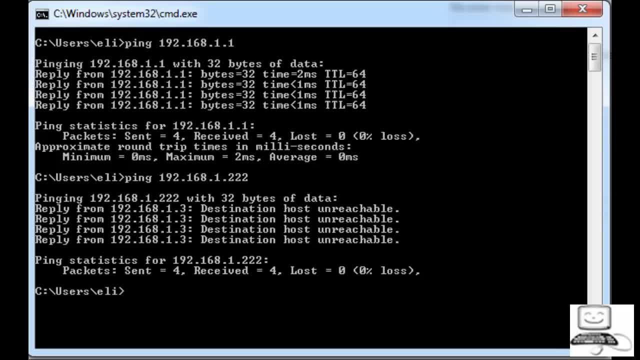 see that the host is unreachable, or we will see that there is no reply at all. so 192.168.1.1. we saw that it what that that computer, that device was accessible. then when we go and do the other one, we see it is not accessible. 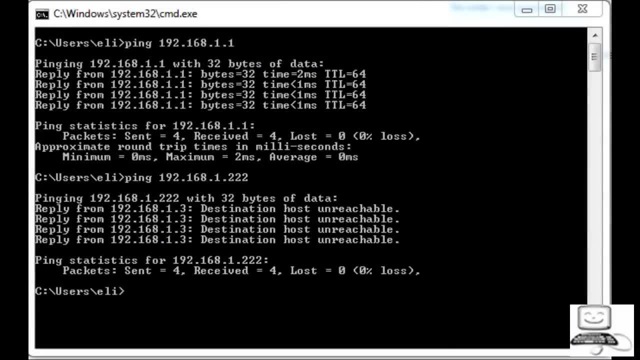 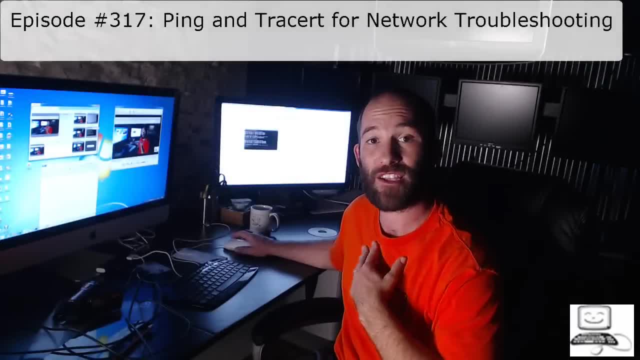 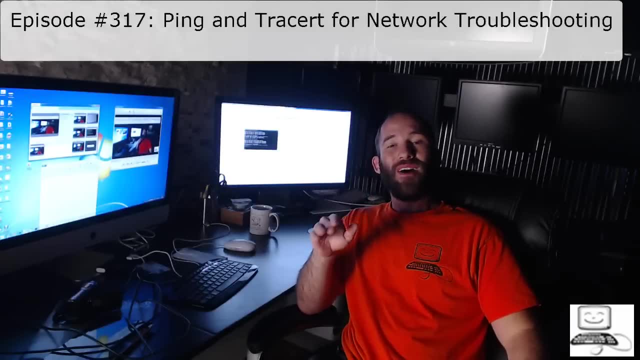 that is basically all the ping command is, though. it pings the network device or computer, and then the network or device computer responds back to you to tell you if it is active or not. now there are two reasons that a computer or network device may not respond back to you. the first one, obviously, is that it is off or it is. 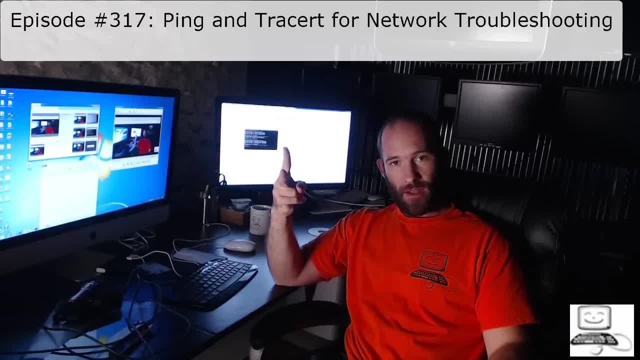 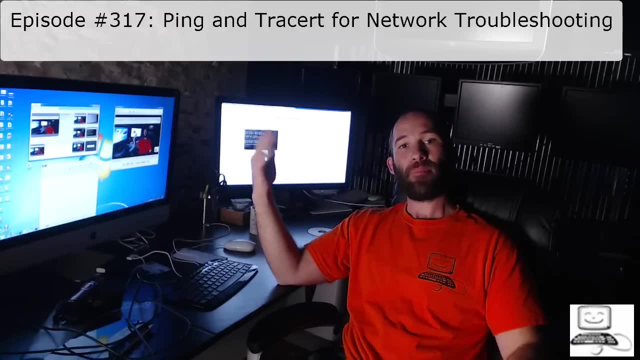 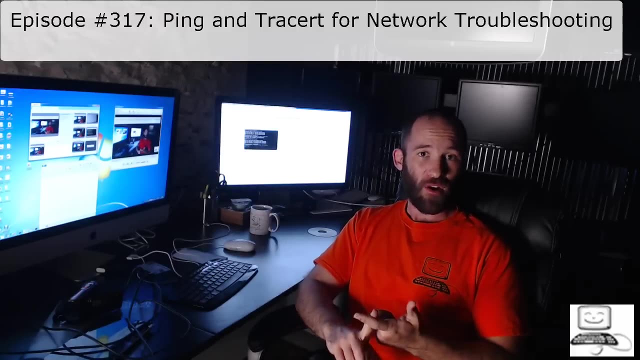 broken, so that's a problem. the second one is that if it has been configured not to reply to ping traffic- this is the ICMP traffic- if it has been told not to do that, maybe it has a Norton firewall installed or McAfee firewall installed. so that is one. 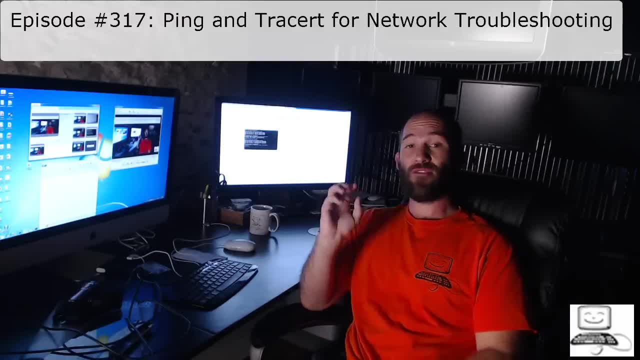 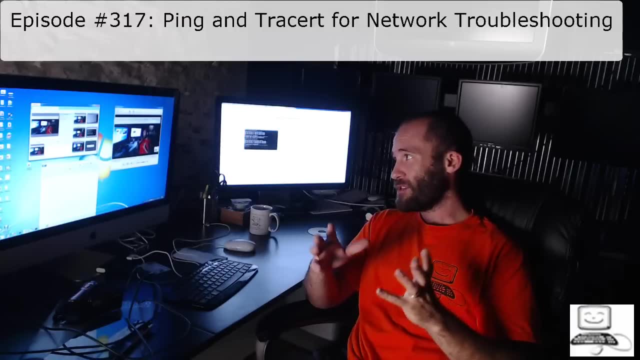 thing that is important to understand is that it's been configured not to respond to a ping. then it won't respond to a ping, but most devices in normal networks will be able to respond to this ping. so how do you use the ping in the normal world? well, 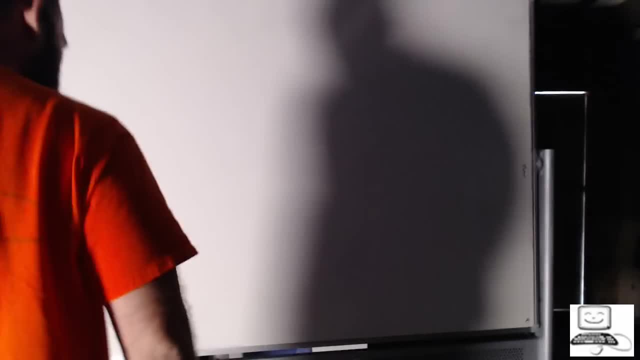 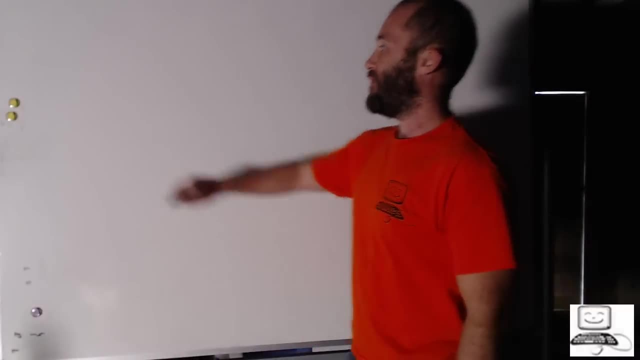 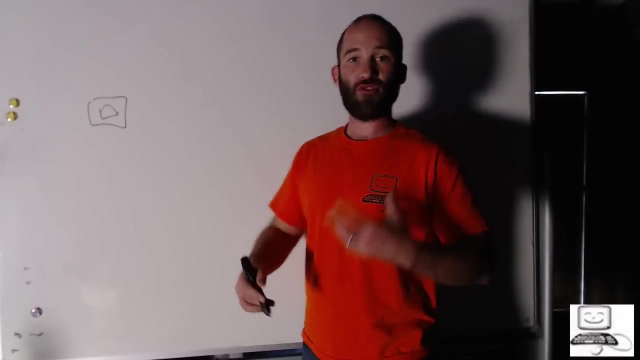 basically how you use the ping in the normal world is you use it to figure out what devices are active so that you can figure out what you need to fix. so if you are sitting at your computer and you seem to be having networking issues, you can use the pink man to try to figure out what is going on. the first thing 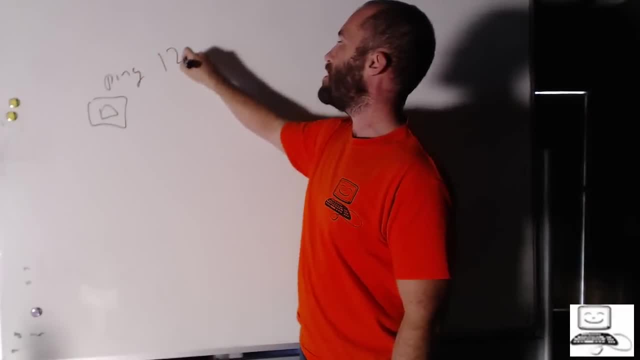 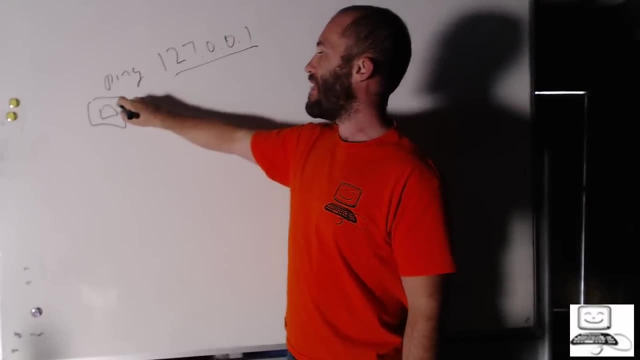 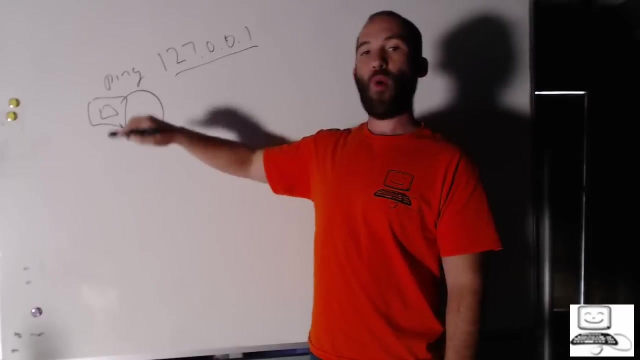 that you will try to ping is: you'll do ping and you'll do 127.0 doesn't have 0.1. if you ping 127.0 does 0-r-0-1. that is called the loopback address. the loopback address is the network card itself. so essentially you are pinging. 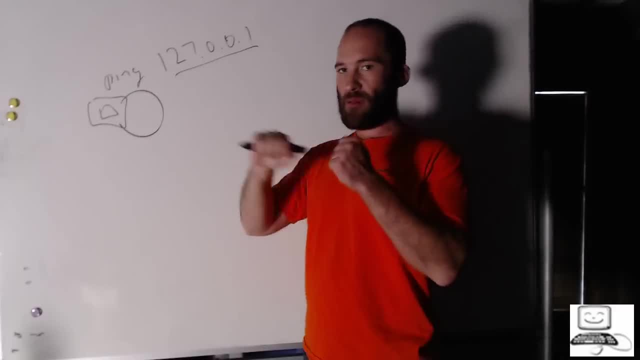 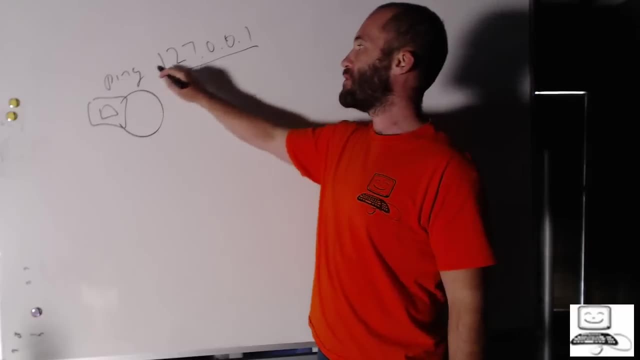 yourself from yourself, so you don't need a cable attached. you don't know we'd need anything. you could, as long as you have a network card installed and the driver is onalso a solv 눈 everT위 are installed properly, you can ping 127.0.0.1 and you should receive a response. 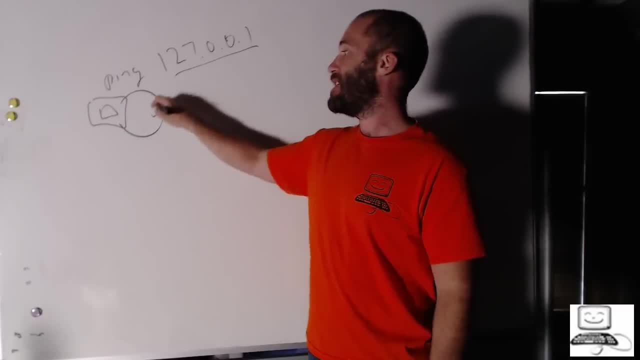 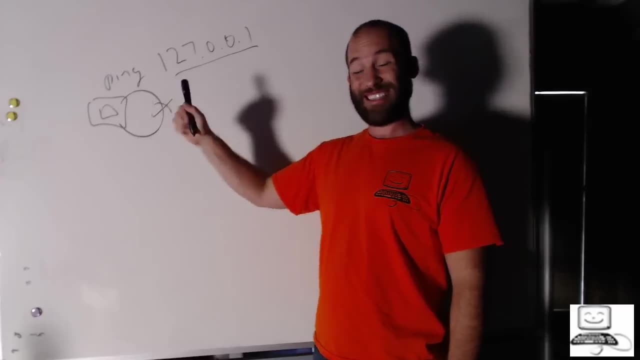 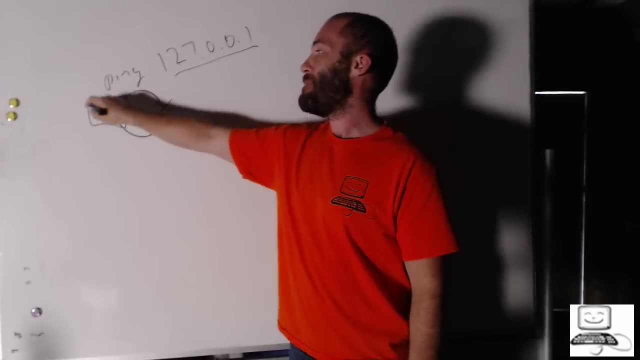 That is A-OK If you don't receive a response. if this doesn't work, that may mean your network card drivers are not installed properly. That may mean the network card itself is dying or has problems. Essentially, if you try to ping 127.0.0.1 and there are any problems, then that means. 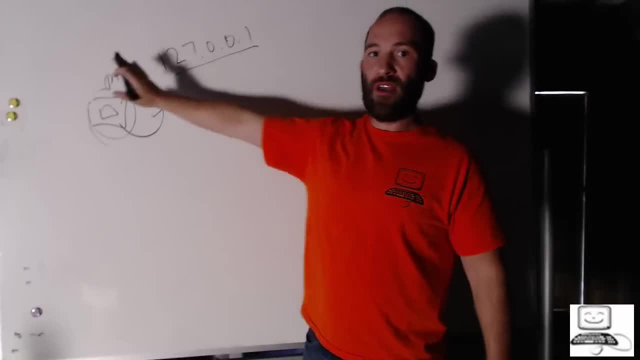 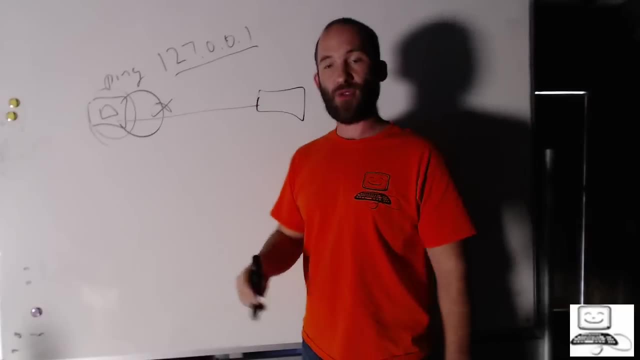 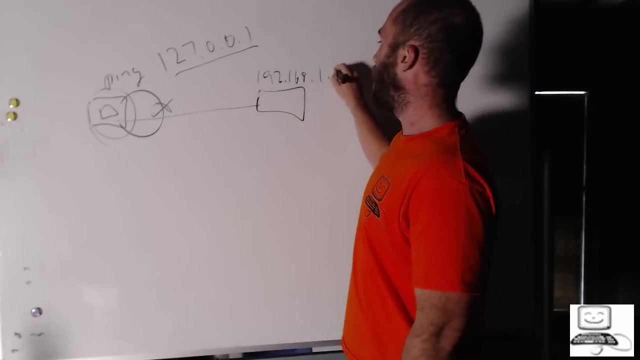 there is a problem with your computer. Look no farther, It is your computer. The next thing that you can do is you can then go and you can ping a device or a computer on the network to see if it is accessible. So I pinged 192.168.1.1.. 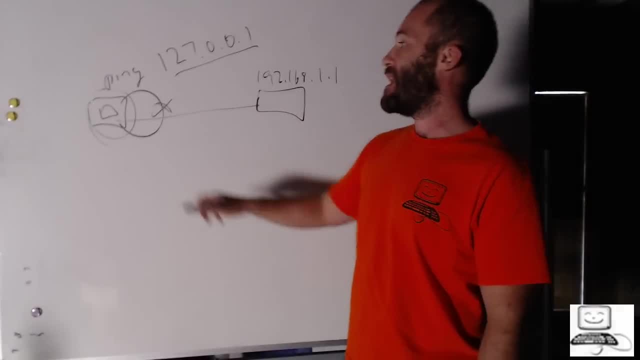 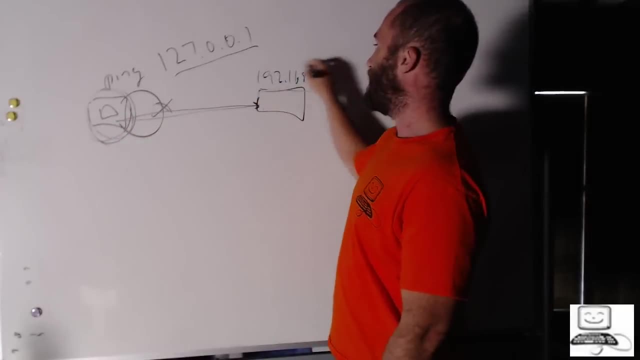 That is the default gateway, That is the router that is sitting on my network. So the question is: OK, I know my network card is working, so now I'm going to ping out and see if this device responds. Now, if this device does not respond, you know that there is either a problem or there is. 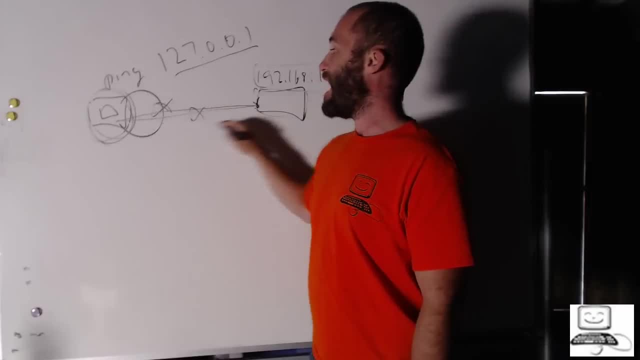 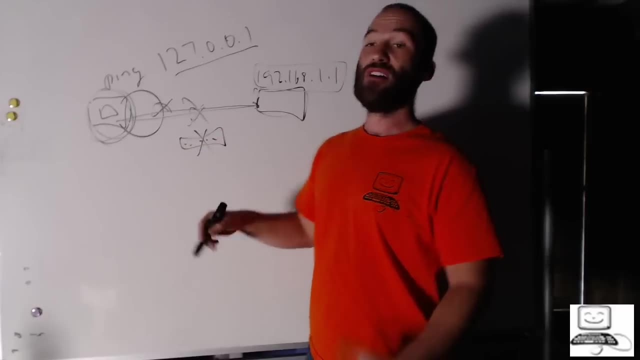 a problem with this device, or there is a problem with the connections in between. Maybe the cable has been cut, Maybe the switch that is connecting everything is powered off, So on and so forth. So, basically, what you do is you try to ping something that you know should be active. 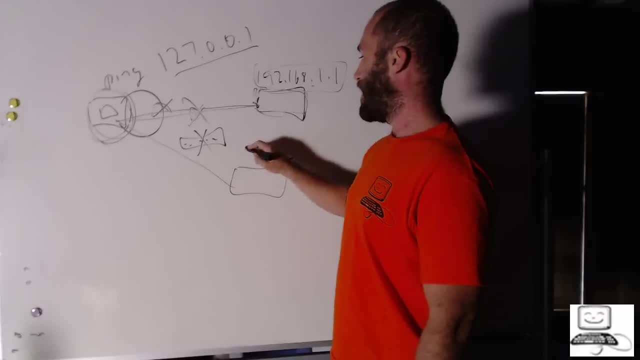 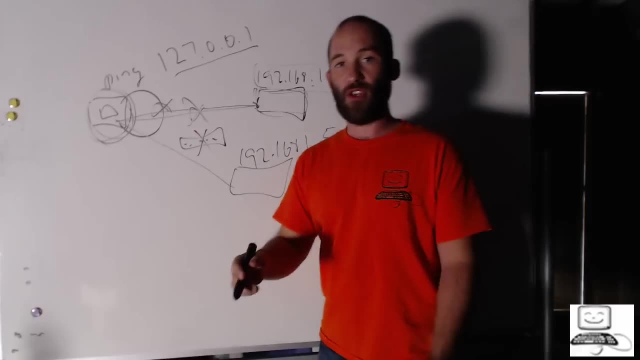 If that doesn't work, you then try to ping another device. So let's say you have a printer on the network. 192.168.1.5.. This would be an IP address that you already know. Now, if you try to ping this device and it doesn't work and then you try to ping this, 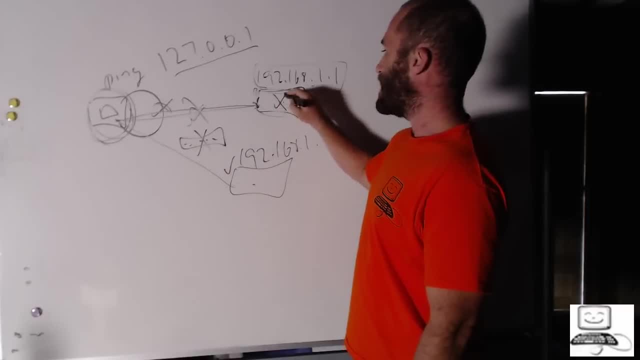 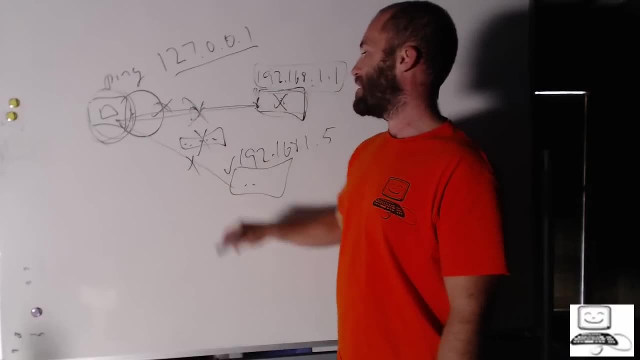 device and this does work, then you know that there is an issue with the first device. If you try to ping this device and it doesn't work, and you try to ping this device and it doesn't work, then you know it's probably the cabling, the switches, some part of the. 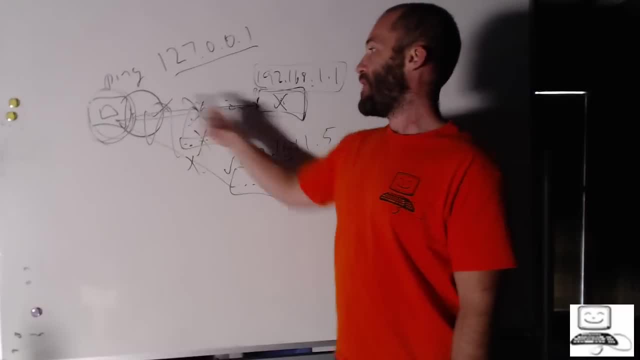 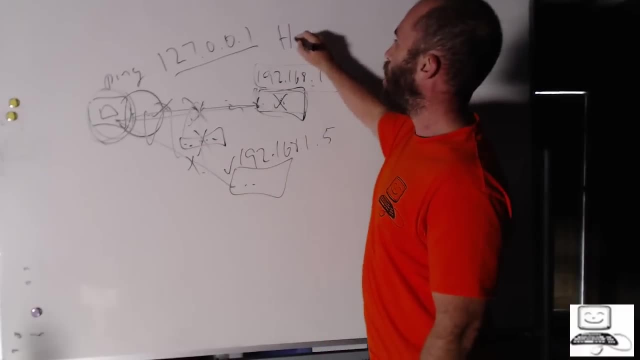 networking between the devices. So that's how you troubleshoot that. The next thing you would do is you would ping a device or the computer. You would ping the computer by its host name. So this is the friendly name you have for a computer. 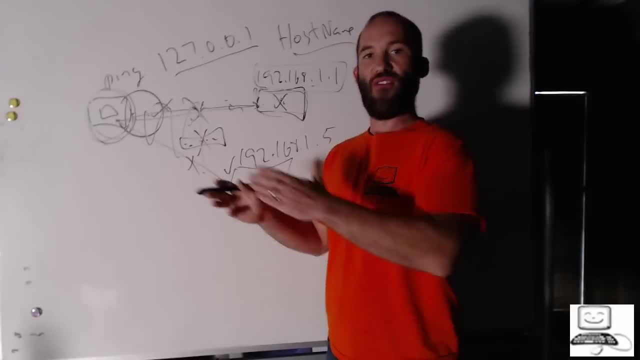 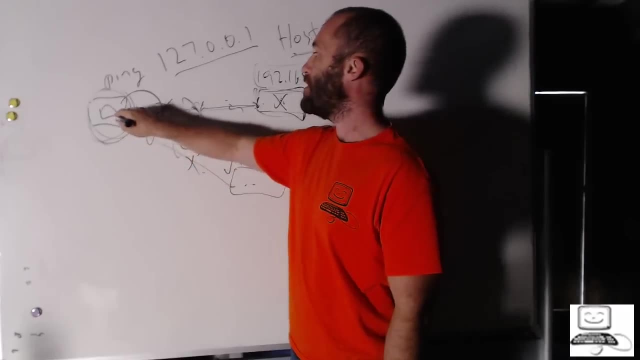 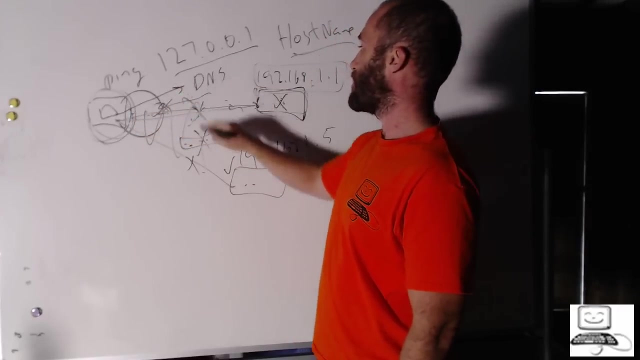 So Eli's laptop server, file server, whatever you have called the computer, is the host name. Why that's important is because what will happen is your computer will make a call to DNS and will try to receive back the IP address of the computer you're trying to access. 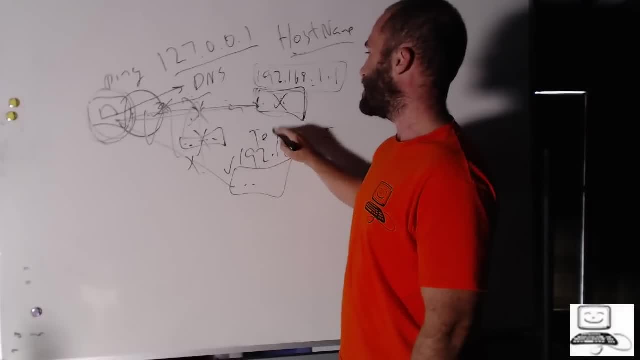 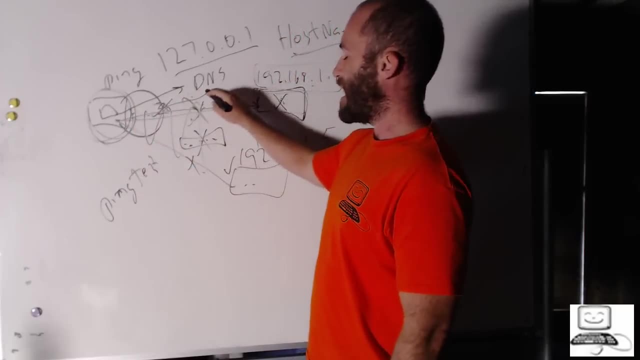 So 192.168.1.5 is called test. We can do ping test. That will call out to the DNS server. What you'll see, I'll show you in the example, is you should get a reply that says pinging. 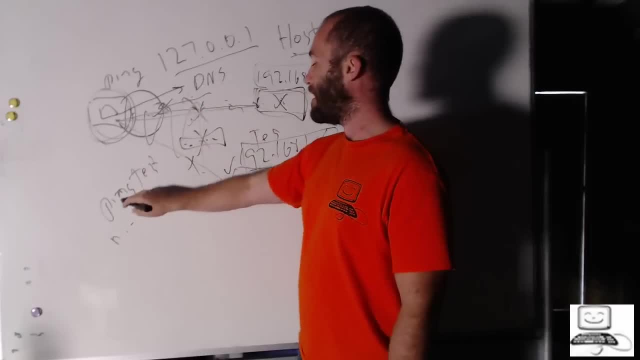 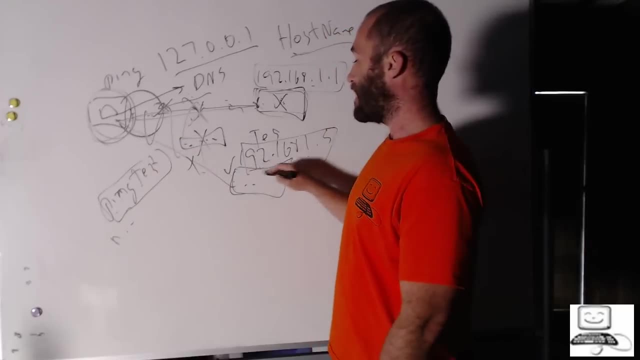 the IP address. So it should resolve the IP address and then ping the computer. Well, if it resolves the IP address but then can't talk to the computer, you know that there is an issue here If it doesn't resolve the domain name. If it doesn't resolve the domain name at all, it can't turn the domain name into an IP address- then you know that there is an issue with your DNS settings. Most of the time you see this when somebody has gone in and messed with the network card. 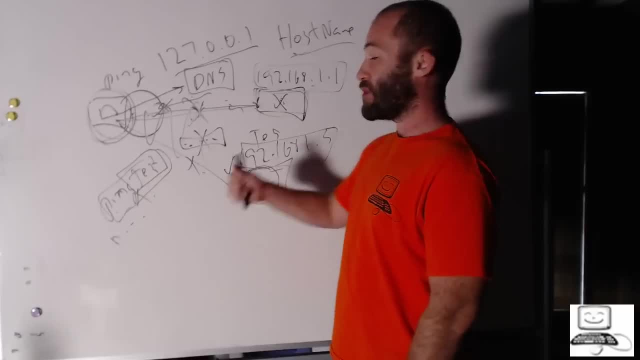 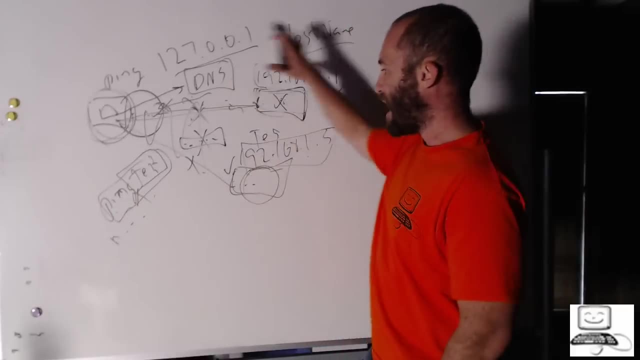 and changed the DNS settings. So if you try to ping the IP address, it works fine. When you try to ping the domain name, it doesn't work. Well then, if you're trying to go farther, so now you've figured out your entire local. 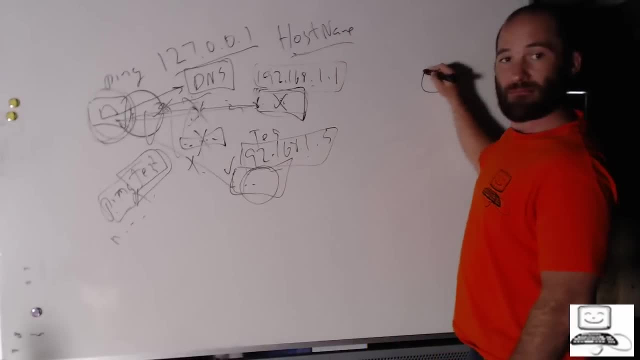 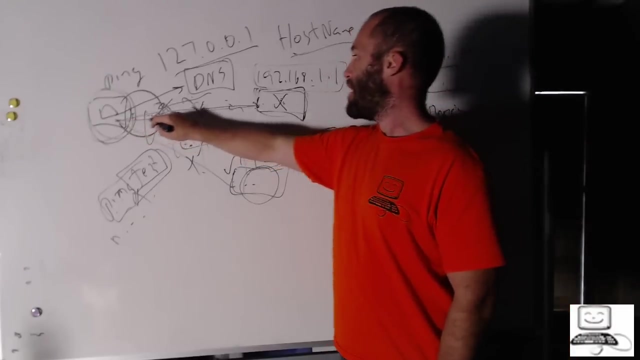 area network works. So now you're trying to figure out about a problem, Trying to get to, let's say, cnncom or, in the example I'll show you in a minute, dslreportscom, because it's easier. So if we're trying to figure out what the problem is here, then what we can do is we. 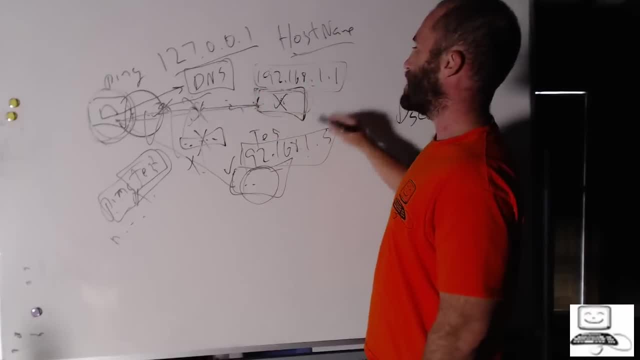 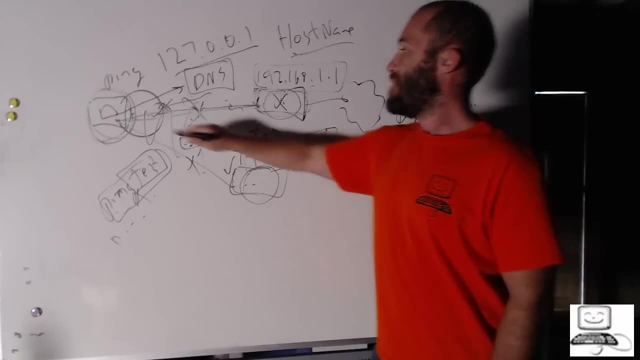 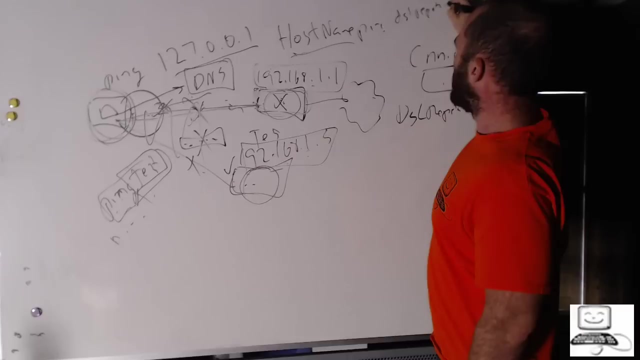 can ping our default gateway 192.168.1.1.. That tells us if we can get to the default gateway that should get us out to the internet. Then we ping ping dslreportscom. Okay, Cool, So dslreportscom. that should resolve to an IP address and then we should be able to. 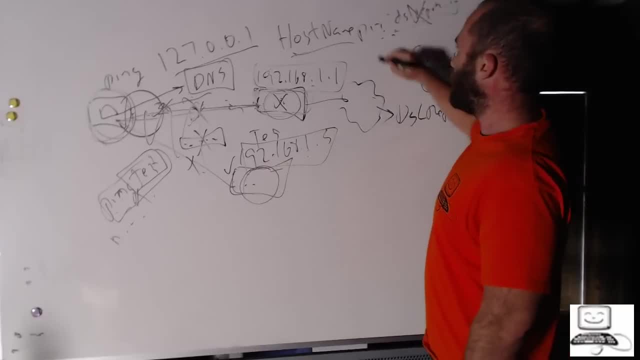 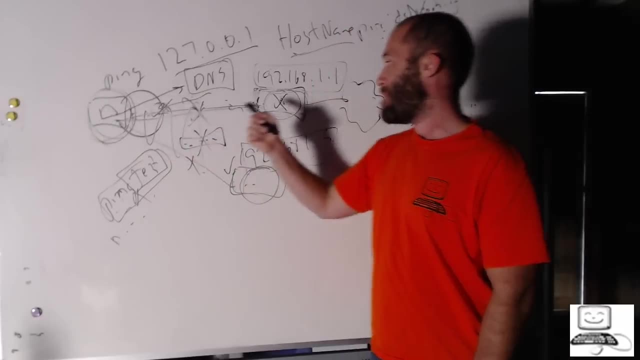 ping it and get a response. If that doesn't resolve, then we know that we have a problem with DNS. Again, it may be a DNS setting in our computer At this point. it may be a DNS setting within the router itself, or if this is your own server. 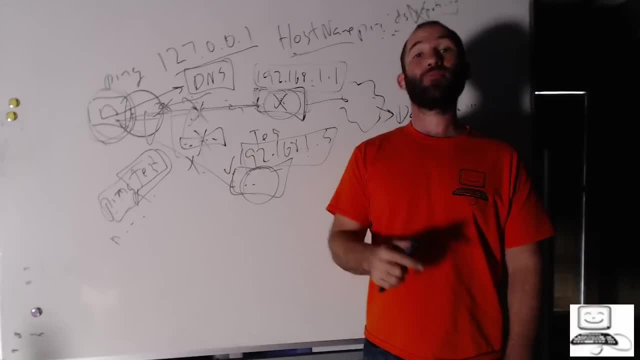 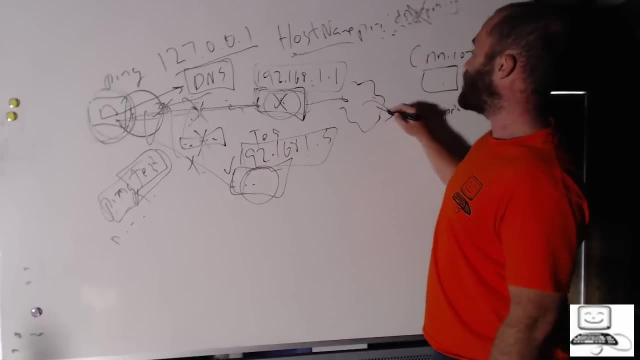 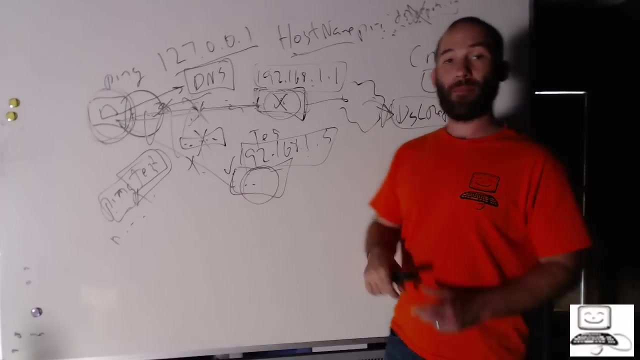 whatever you're trying to ping is something that you've set up. maybe it is a problem within the internet DNS. If you can't ping by the domain name, you try to ping by the IP address for the server. If you still don't get a response, then you know there's probably something mucked up. 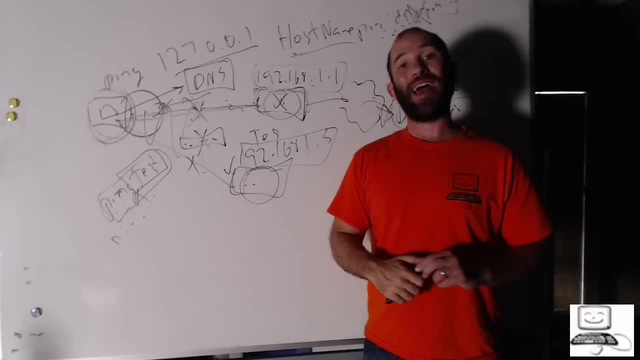 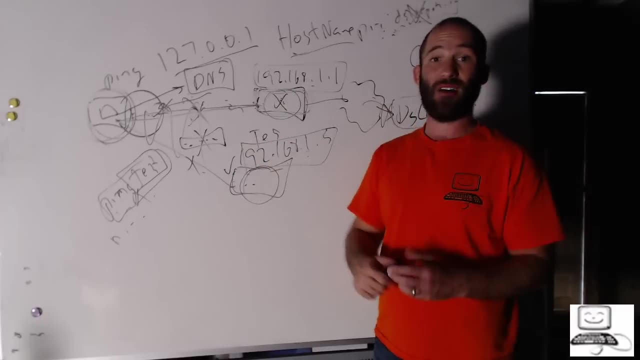 with your server and if you do get a response, then you know it goes back to DNS. So this is the overall process of how you use the ping command for troubleshooting, and I use this all the time. It's very, very useful and it's very, very simple. 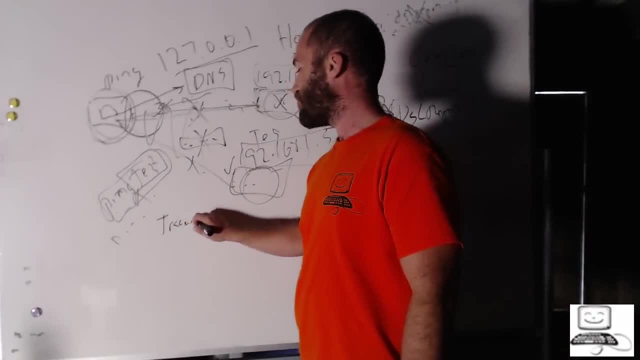 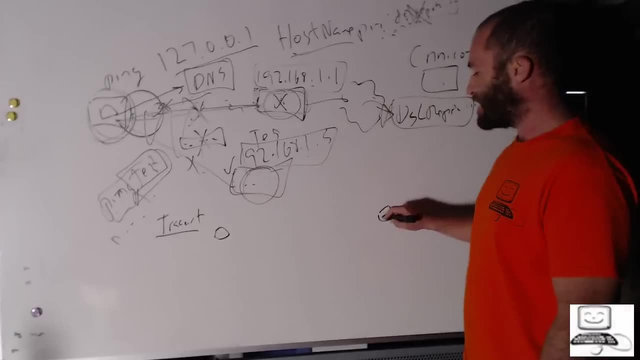 The final tool that I will show you at the end is something called Tracer, TraceRoute or TraceRT. What Traceroute does is when you're sitting at your computer and you're trying to access another server as your packets go through the different hops to get to the server that 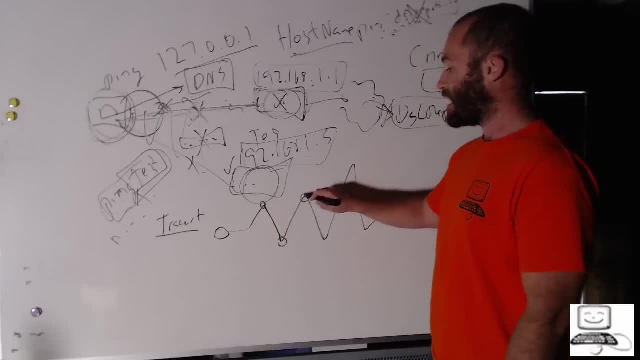 you're trying to connect to. so when we talk about hops, we are talking about routers. it will send a reply back to your computer for every one of these routers. It goes through, the packets go through, so that if there is a problem you know exactly. 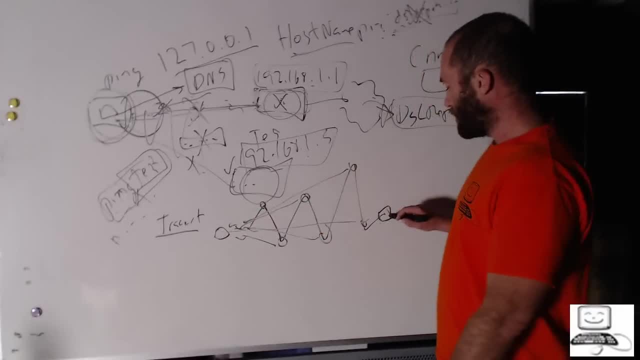 where the traffic stopped. So if you're trying to go from your computer to this server, you get the first reply, you get the second reply, you get the third reply and then, let's say, on the fourth one you don't get a reply. 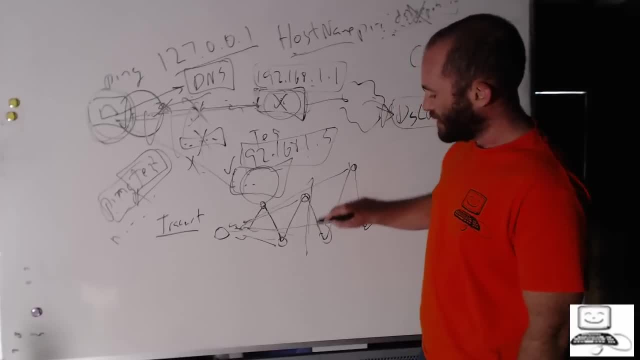 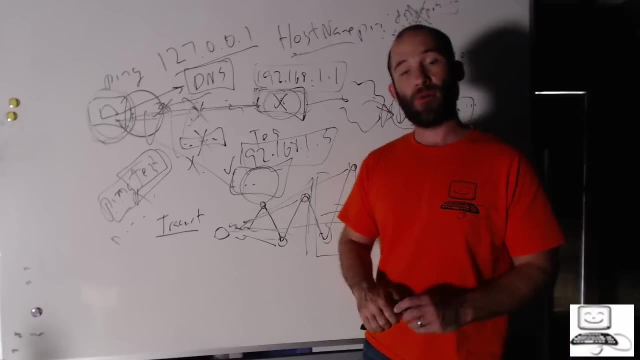 Well, you know, all the way up to here, the routers work, and then there's an issue somewhere on this side It shows you where the traffic stops. This becomes important especially in the modern world, where more people are using co-location facilities. So co-location facilities are where you take your own servers. You put them into a data center. so you rent space in a data center. Well, if you're having problems accessing that server, you don't know if it's you, you don't know if it's your ISP, you don't know if it's a co-location facility's networking. 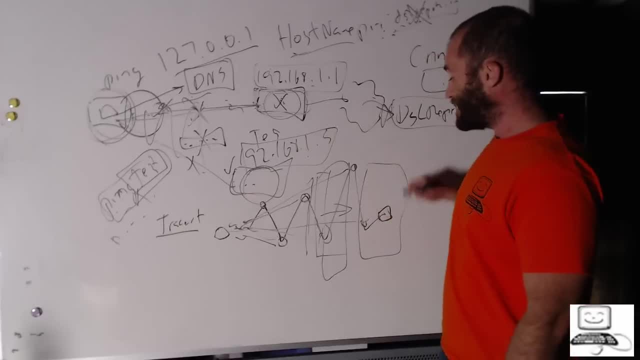 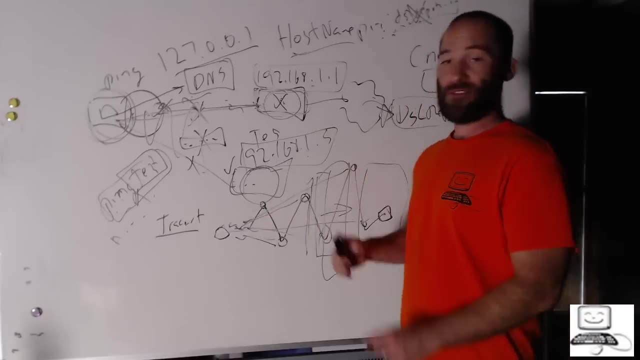 equipment- or maybe it's your networking equipment- that's sitting in the co-location facility. Using the trace route command will allow you to try to figure that out. I used this quite a bit back when I had my server up in the co-location facility. 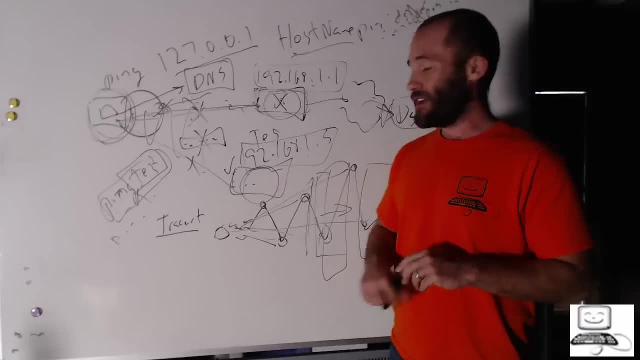 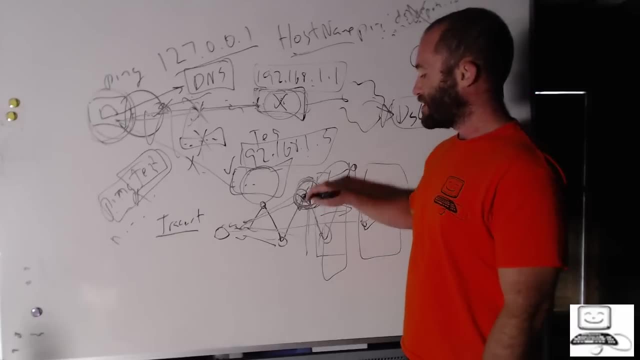 Sometimes it was my fault, Sometimes it was a co-location facility's fault. By using the trace route command, you can go. oh, I know that this is the last place that the communication was seen, so I know whoever controls this router is the one that. 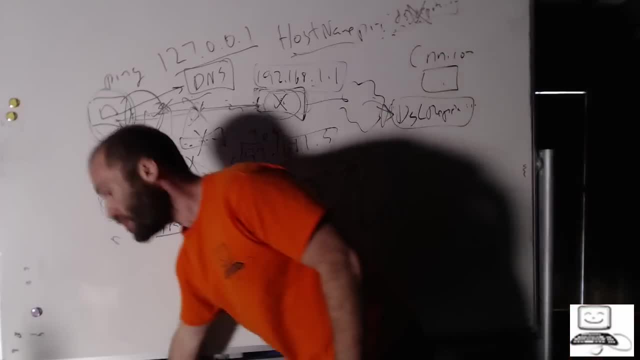 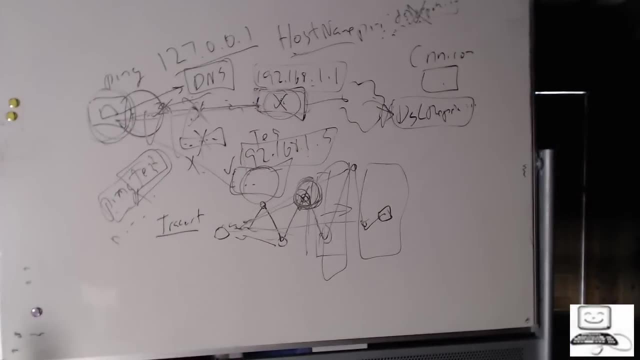 needs to make the repair. So with that, let's go back on the computer and I'll show you how the ping command works. So let me make sure my Windows 8 computer is up so that I can actually in fact ping it. 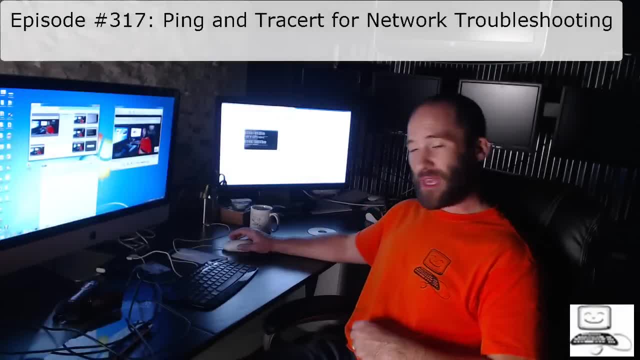 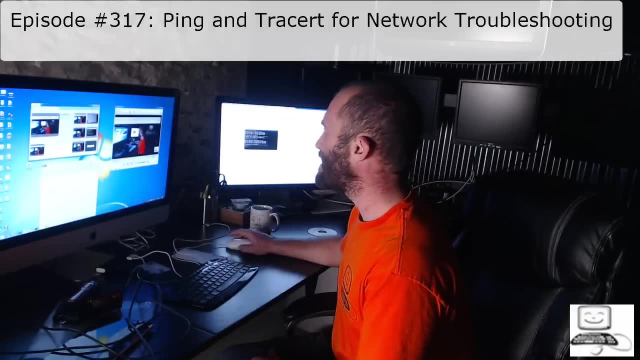 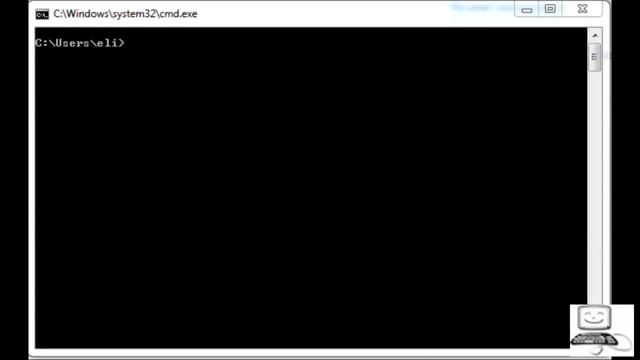 Okay, So this is just a normal Windows 7 computer, So ping works on Windows 7.. Hopefully it'll work on Windows 8, Windows Vista, Windows XP, Windows 95, Windows NT, so on and so forth. So let me just put a screen there and we will go to the screen. 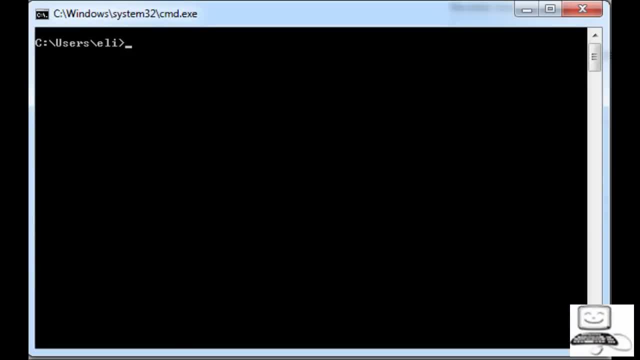 So here we are just sitting at the command prompt. So this is just a normal command prompt that you go to. As I showed you before, if I want to ping my router, I do 192.168.1.1, and then I'm. 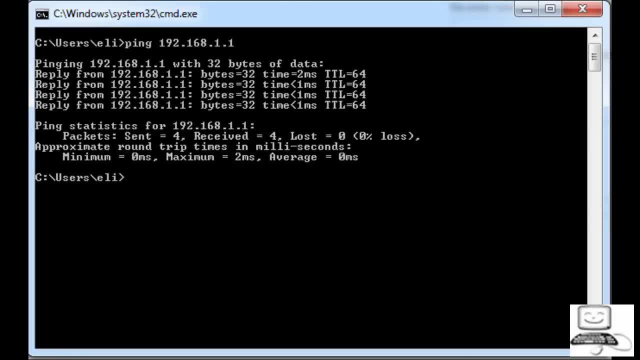 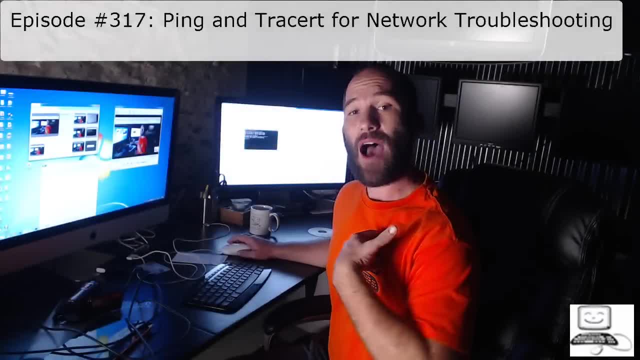 going to ping my router And that pings my router and tells me that my router is working. Now the question that you may have. you say: okay, well, Eli, you know what your router's IP address is. How do I know what my router's IP address is? 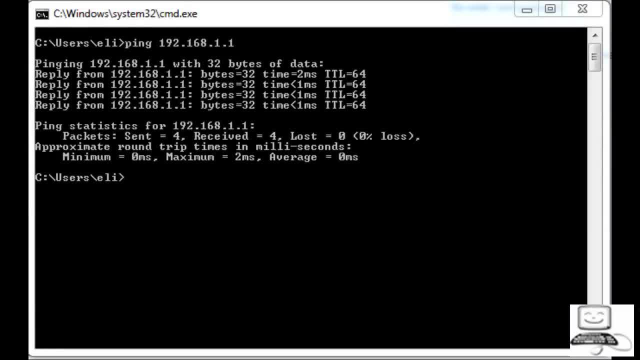 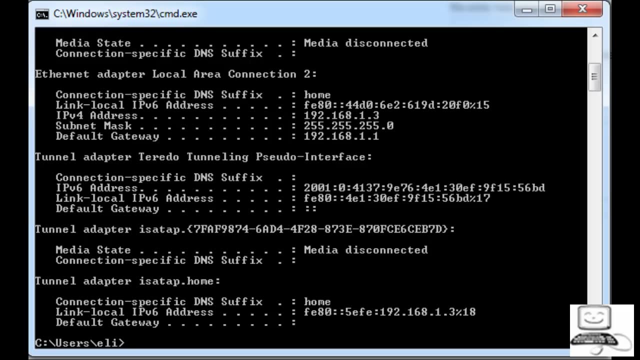 Well, that is where you can use the ipconfig command. So ipconfig, that's all it is, and this will give you your IP configuration settings for your computer. So I hit enter And then, if we can see, let me get my little drawing thing. 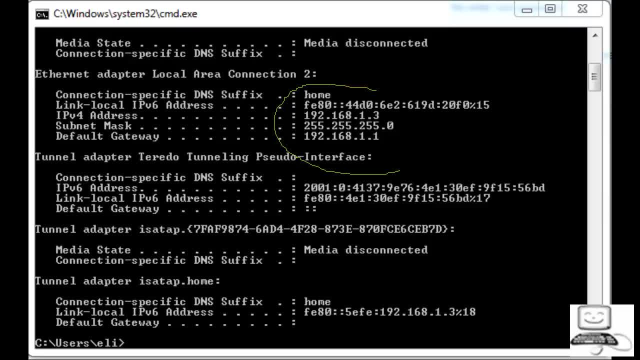 So, if we can see up here, this tells us the information about the network card that we're dealing with. So you can see that the IPv4 address is 192.168.1.3.. So that is the IP address of my computer, of this computer. 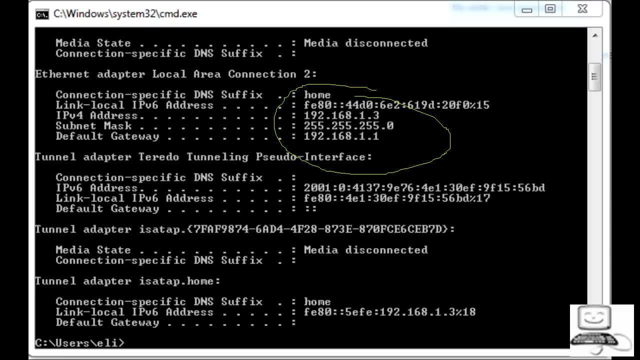 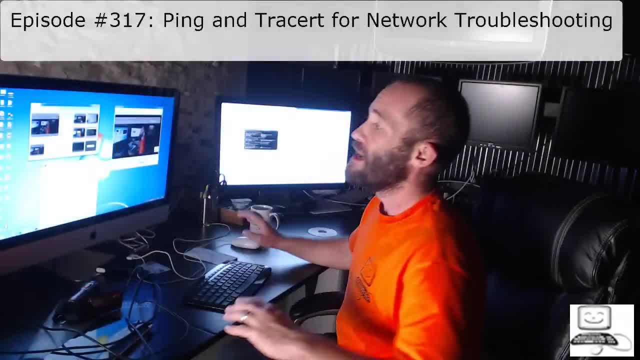 The subnet mask is 192.168.1.3.. The subnet mask is 255.255.255.0.. And the default gateway is 192.168.1.1.. So it's important that you understand a little bit about these TCP IP settings. 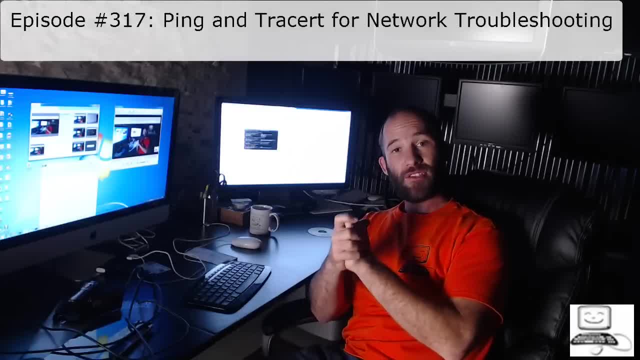 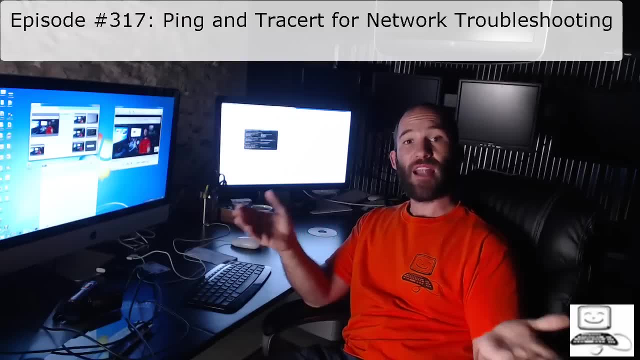 Remember, these are generally all received from the DHCP server, so they may be different from you. You may be 192.168.2.1.. Or you might be 10.1.10.1.. Depending on whatever your DHCP is configured for. that is the information you will see. 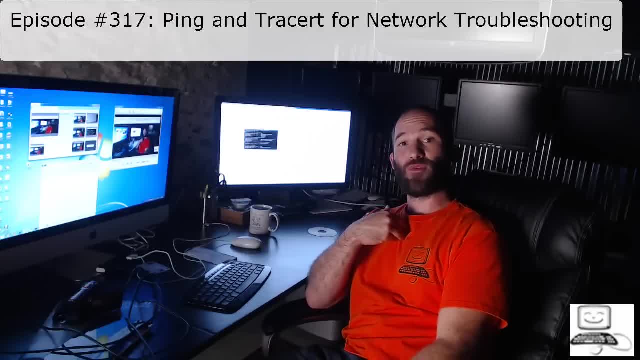 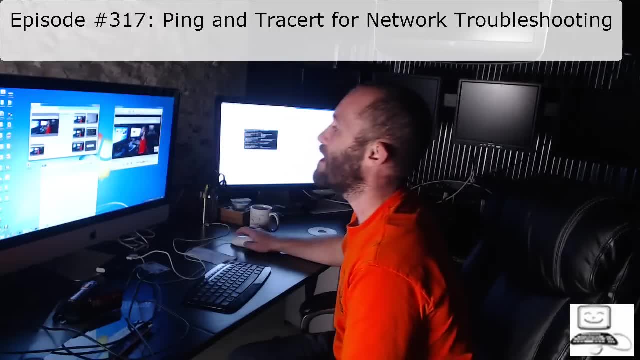 So I'm going to hit enter And you will see there. So just because I say my router is 192.168.1.1,, that doesn't mean your router is that? So do ipconfig so that you can see what the router is. 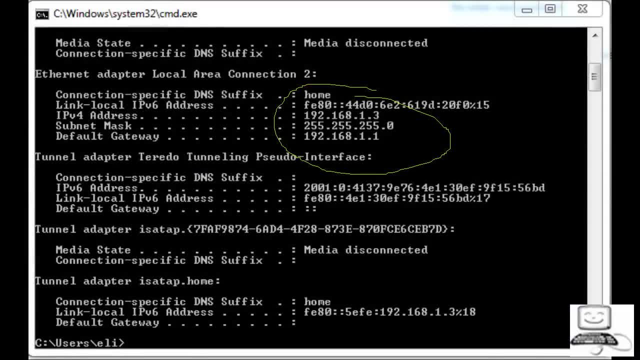 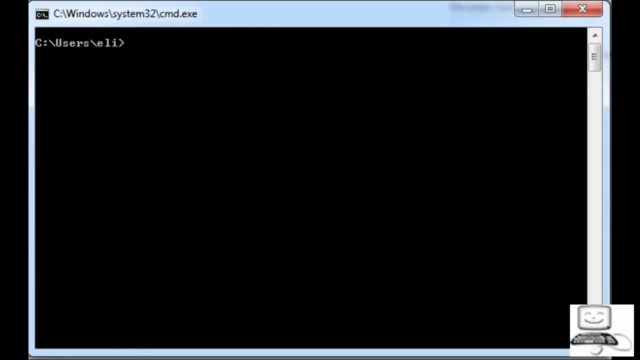 So I can see my router is 192.168.1.1.. So now that I have that I can go and I can just see some of the basic things going on with my network. So if I say, hey, can I talk to another computer on my network. 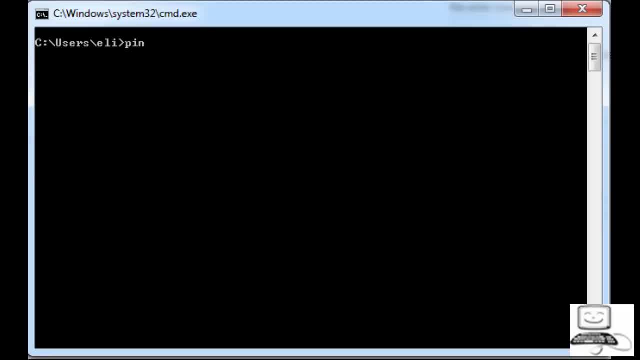 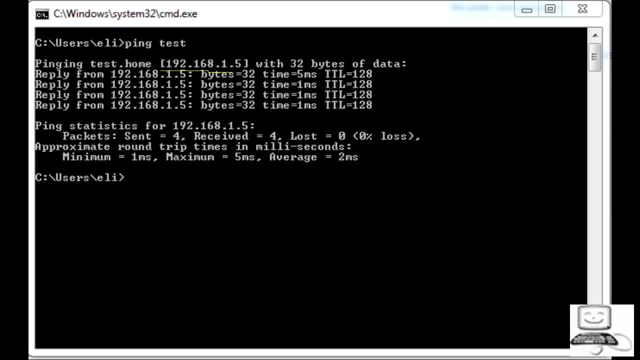 Is DSP working? Is DNS resolving properly? I can do ping and test. So test is my Windows 8 computer. By ping test you will notice that it resolves the domain name. So if you look up here it says ping test. 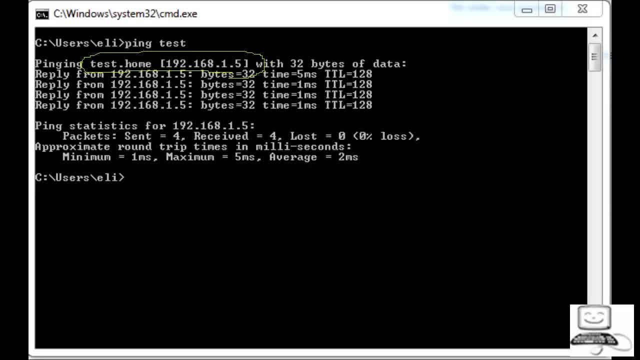 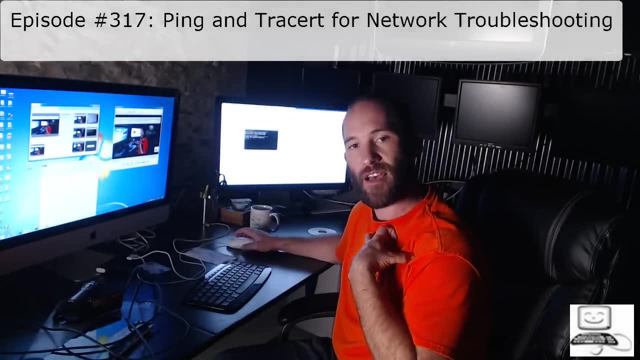 And then it gives an IP address. See, it says pinging test And then it says 192.168.1.5.. So it's showing me That is going out to the DNS server. It's receiving the IP address from the DNS server for the computer named test. 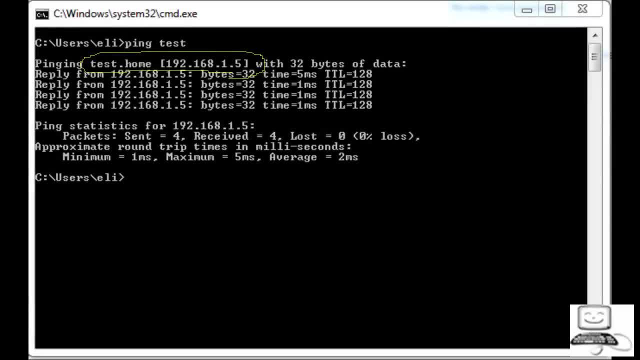 And then it's pinging that IP address. Very important that you understand that concept And then it just works fine. Then obviously, if the DNS did not work properly, I would have to go over to the other computer, find out what its IP address is. 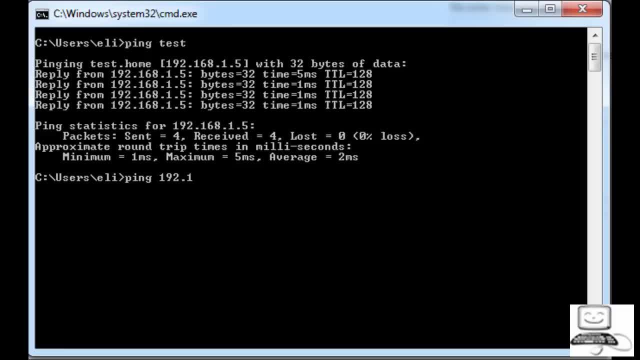 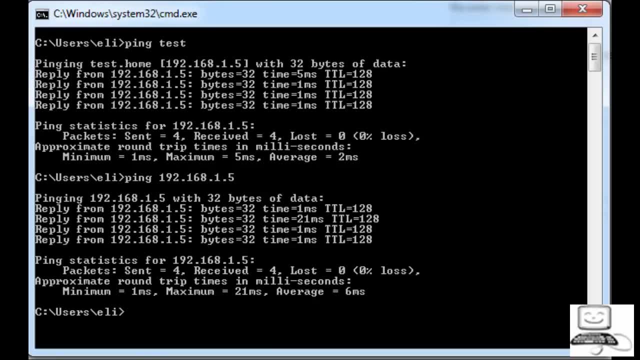 And I could just ping it by its IP address: 192.168.1.5.. 192.168.1.5.. To see if it works. So sometimes if you try to ping by the domain name, that won't work. 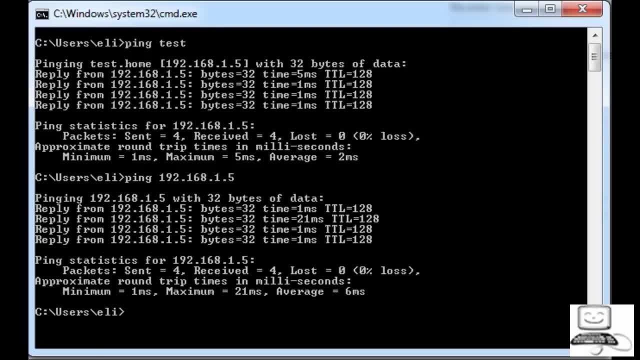 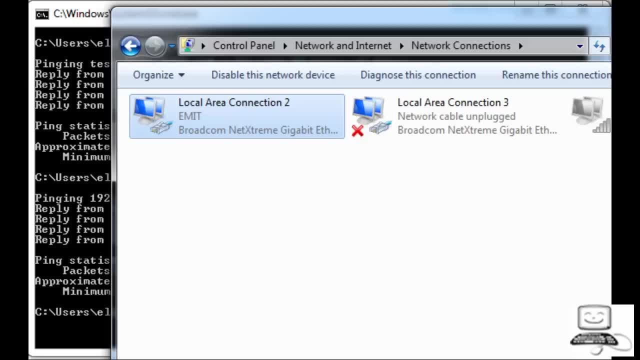 But when you try to ping by the IP address, it will. So therefore, you know that there is a DNS issue. There's a problem with the DNS. Now, when I'm talking about the DNS issue, basically what we're talking about is we go? 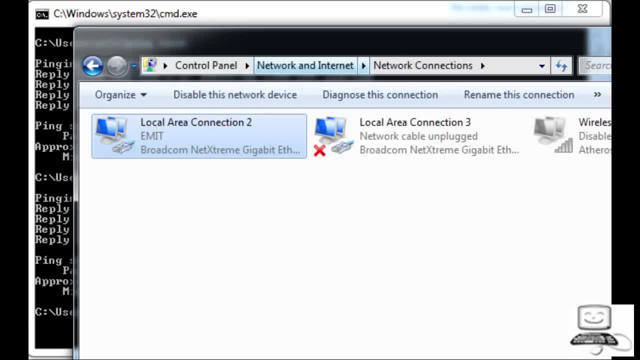 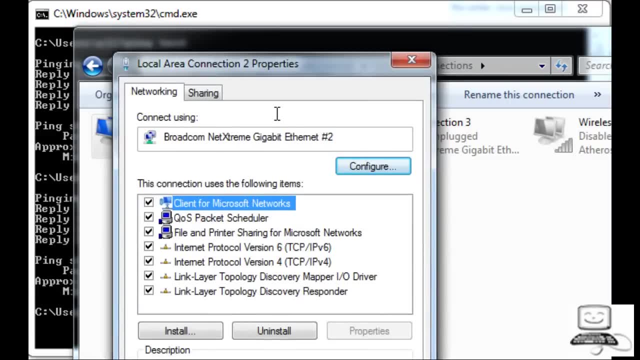 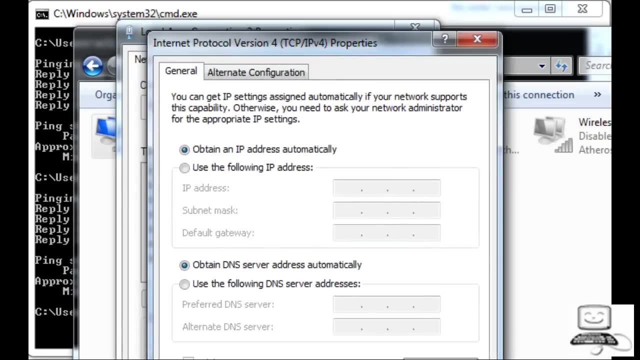 here We go to your network internet network connections. You right click, You go to properties. You then select On TCP IP version 4, and you go to properties And what you'll notice is this gives you how your IP settings for your computer are set. 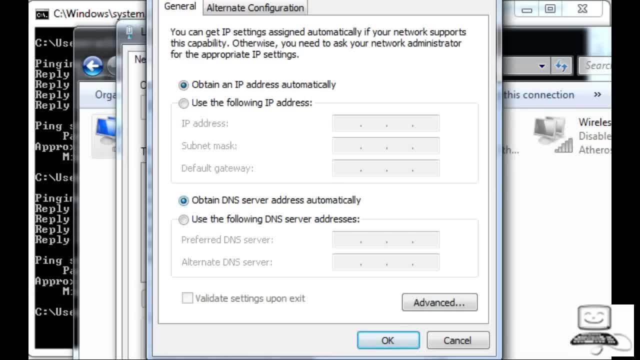 up. Now down at the bottom, this: obtain DNS server address automatically. A lot of times people will have this filled out with garbage. For whatever reason, they will go in here and they will put in garbage. They think that they're being funny. 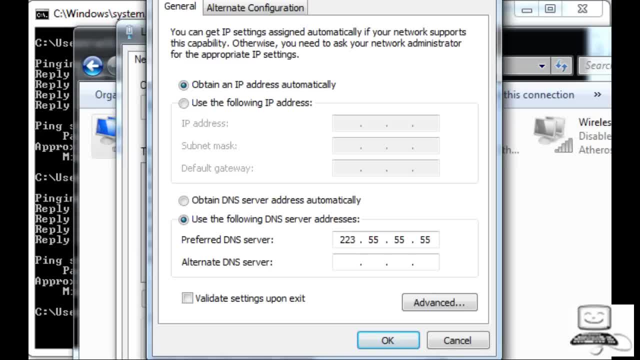 They think they're being cute And in reality they are just messing everything up. This is the server that your computer will go to to resolve an IP address. If the server information in here is incorrect, then it's not going to resolve properly. 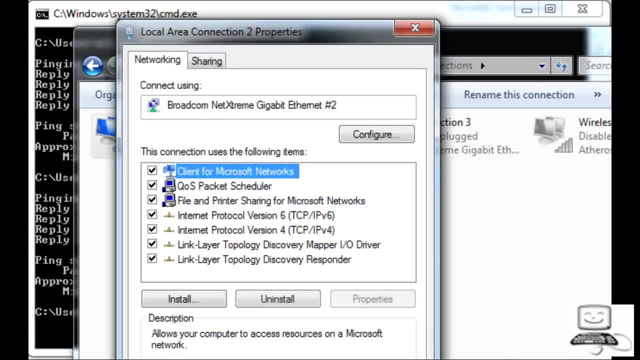 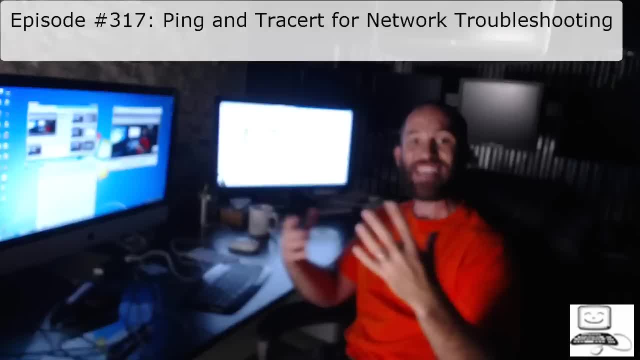 And then you will not be able to resolve domain names. So if your DNS isn't working properly, you can ping by the IP address, but not the domain name. Test CNNcom. Any of those human-friendly, readable domain names you won't be able to see. 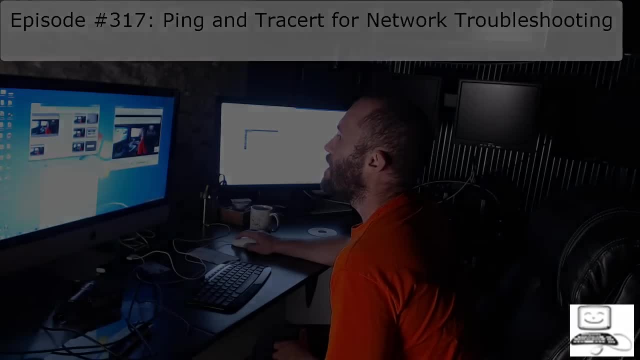 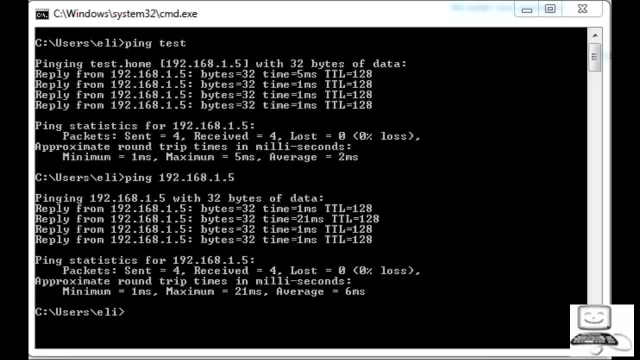 So with that, let me close out of that Bye. And so now we have pinged, So we've pinged the router and I've shown you how to get the IP address for your router. We've pinged the local computer and we've pinged the IP address of the local computer. 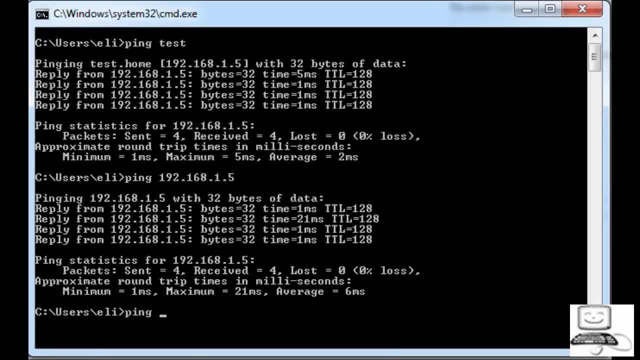 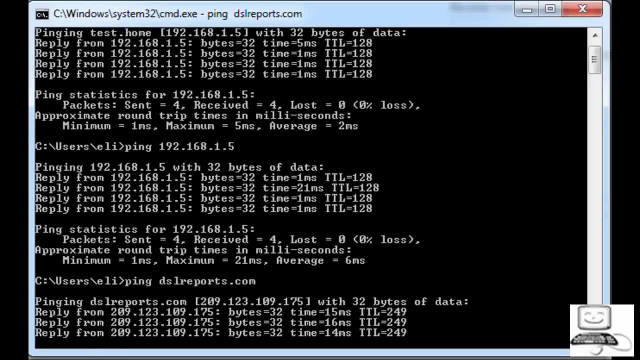 Now what I can do is I can go out and I can try to ping a website such as DSLReportscom. So by pinging DSLReports, this is now out on the internet. This is out. This is all happening out on the internet. 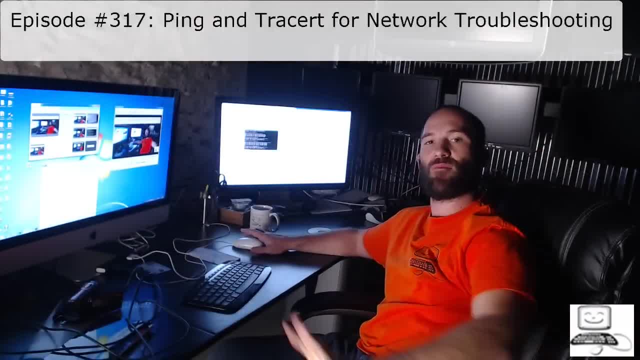 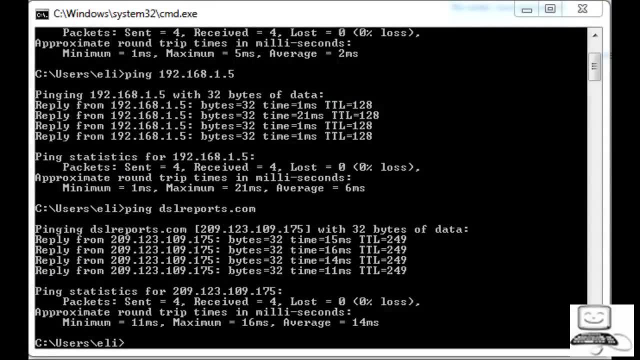 So you're pinging out to DSLReportscom, DSLReports. who knows where that is Somewhere on the cloud. So if this gives you back the proper information, then you know that your internet DNS is working properly and that the server is up and running. 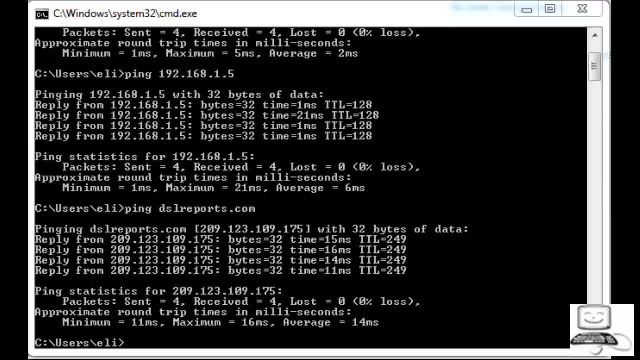 If you can't ping DSLReportscom from the domain name, then you would try to ping it from its external IP address. So we do ping 209.123.109.175, and you hit enter and that will give you a reply. 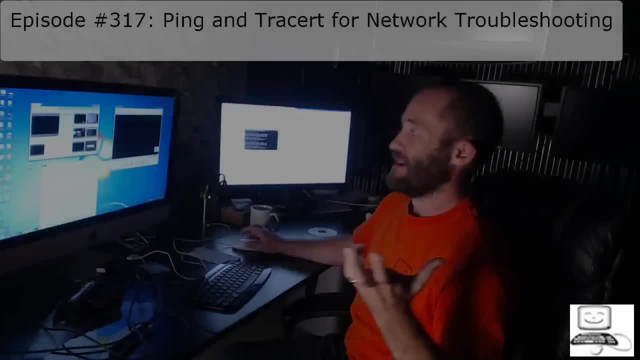 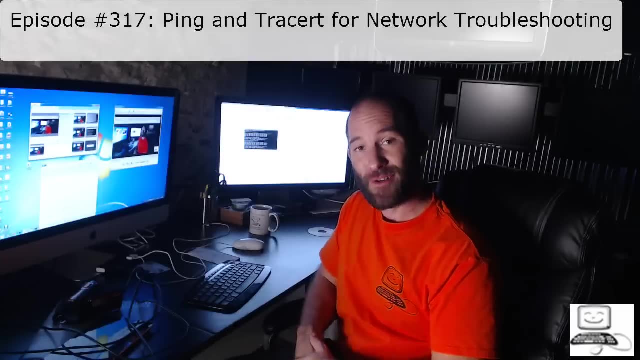 Now why this is important for you is, again, we all want to be thinking about we're troubleshooting somebody else's equipment, but the reality is you might be troubleshooting your own equipment, your own problem. A lot of you guys want to be setting up your own servers for inside your house. 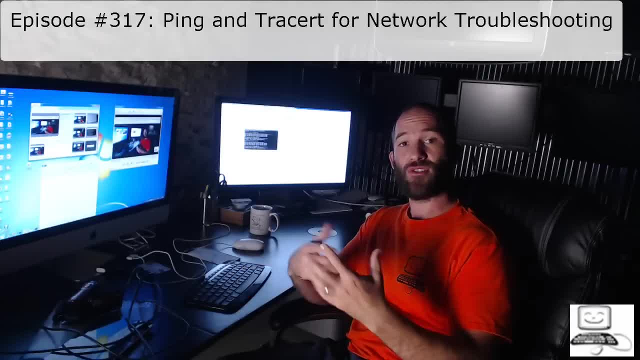 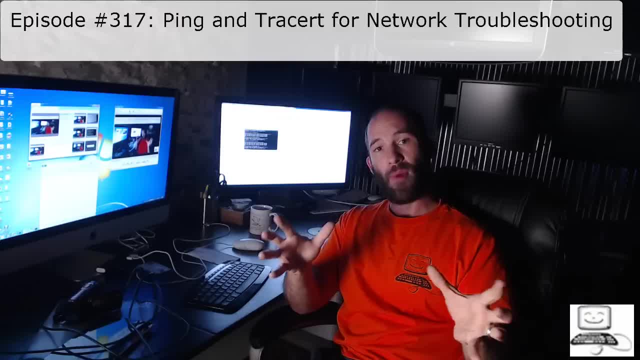 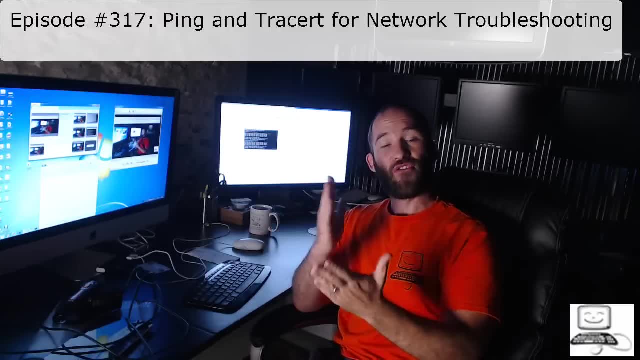 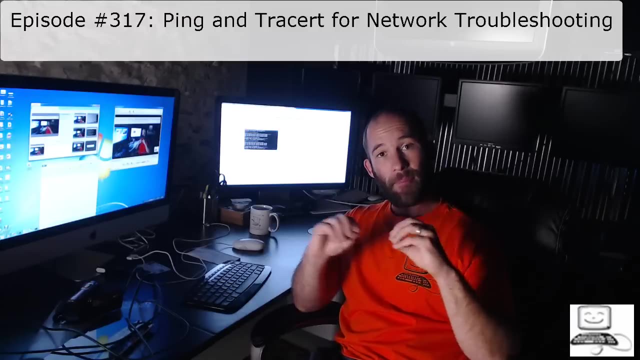 You're not taking my advice. You say, Eli, I want to build my own box and I want to host my own box. So that means you have to go into your own DNS settings from your registrar, so from GoDaddy or oneandonecom or network associates- and change the IP address for the domain name. 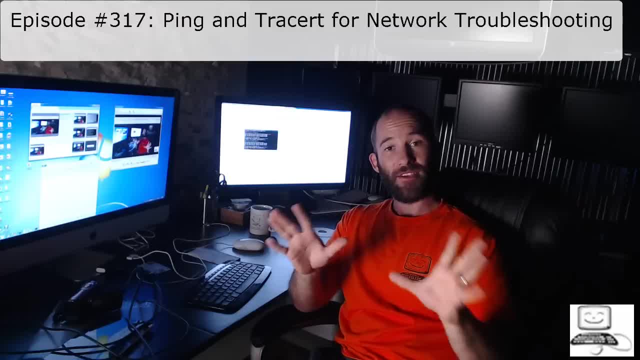 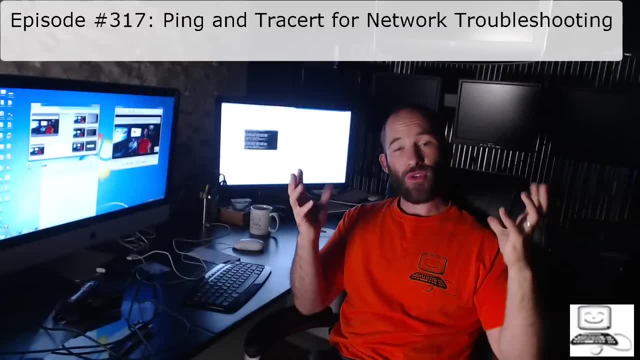 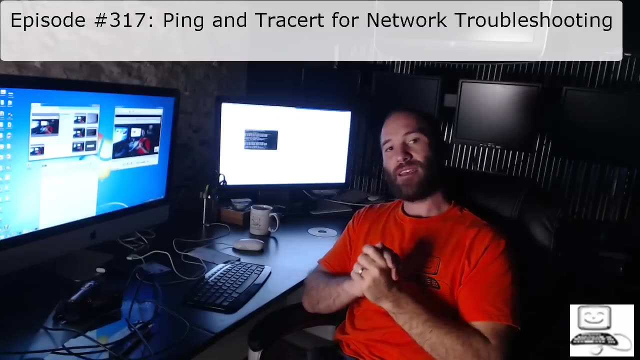 there. If you do it improperly, then it won't work right. So that's where the resolution and the IP address work for this. So that is basically how you use the ping command For troubleshooting. again, it's not too hard, not too complicated, but it is something very 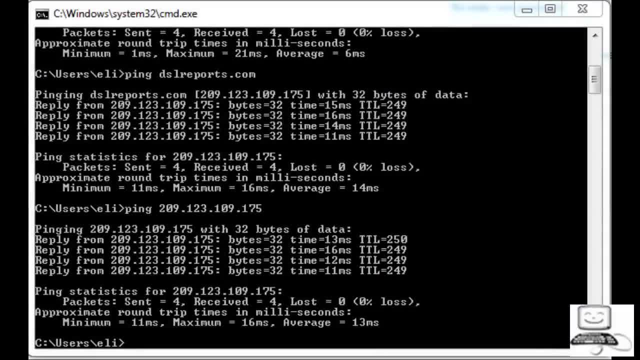 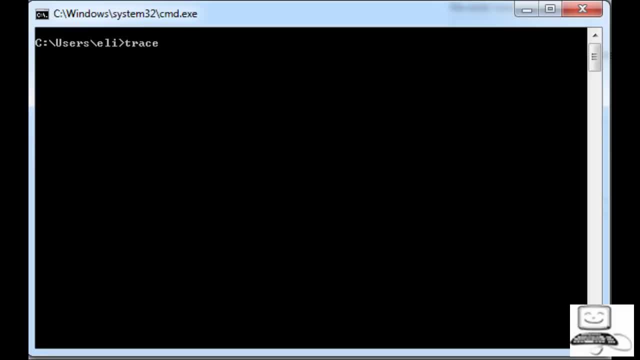 important to understand. Now, the final thing that I'll show you is I'll show you the traceroute command. So I do clear screen, And so what I'll do is I'll do trace T-R-A-C-E route or R-T, so it's just tracert. 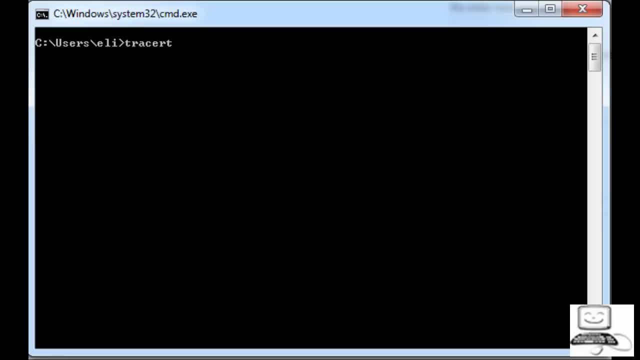 So, me, me, me, I say tracert, but it's traceroute: D-S-L reports, D-S-L reports, D-S-L reports, D-S-L traffic dot com. And then what this will do is this will show you every router that this packet goes through. 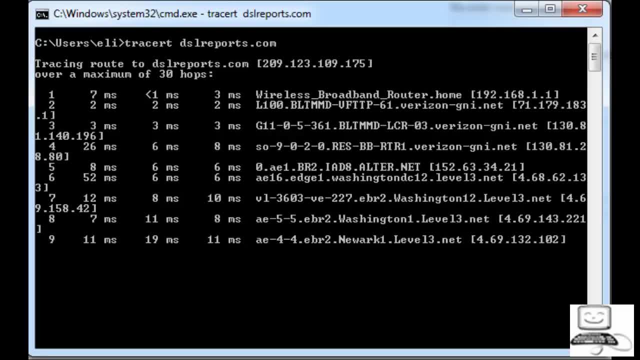 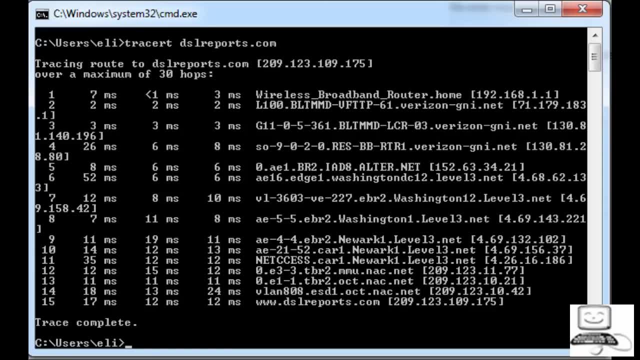 So you will see that it goes through 192.168.1.1,. then on step two it goes through Verizon, then step three, it goes through another Verizon. step four, another Verizon, then alternate, and Washington DC, then Washington DC, then Washington DC, then Newark, then Newark. 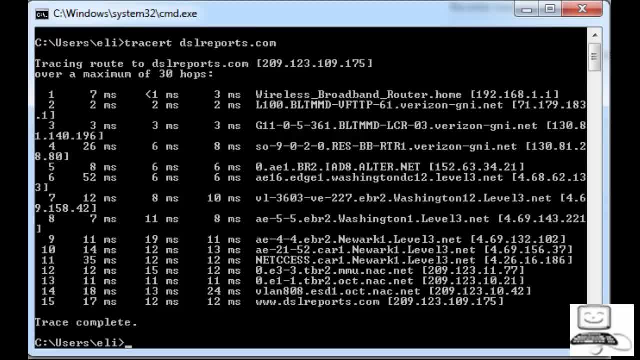 These are all the different routers that the packets go through through in order to get to the final destination, so I could see if, if this failed somewhere along the way, I could go. oh look, the last communication was at Verizon, so maybe it is a Verizon's problem again. this isn't the best. 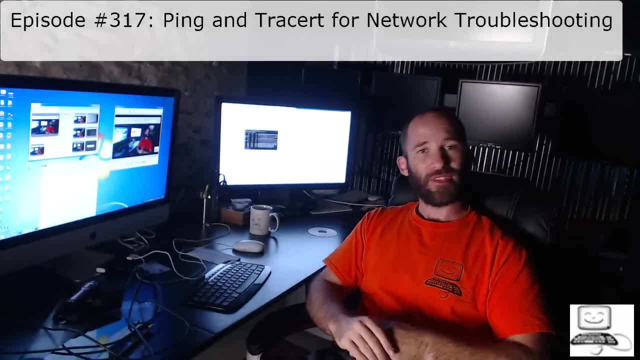 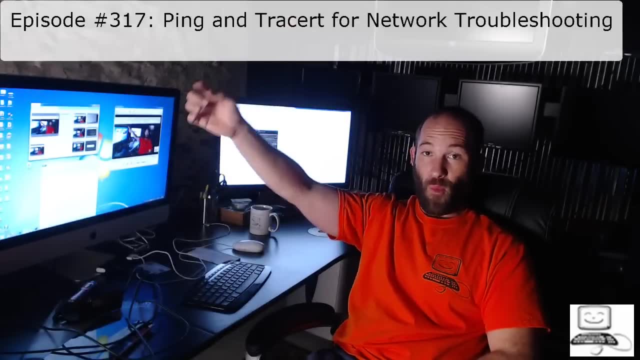 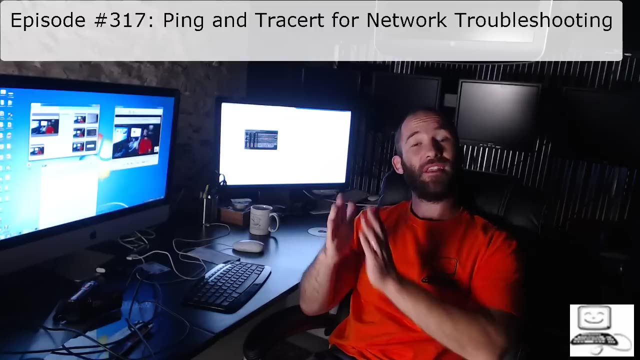 example really here. but I did use it when I have my server in the data center because I could see as the traffic went out of my network, went up to my ISP, went all over the world, went into their, their, their co-location facility and once it went into their co-location facility they had a number of routers there. 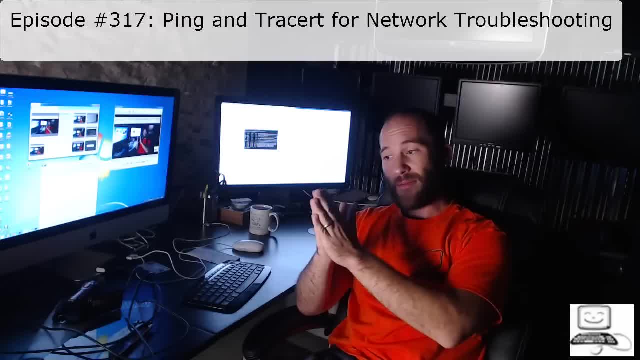 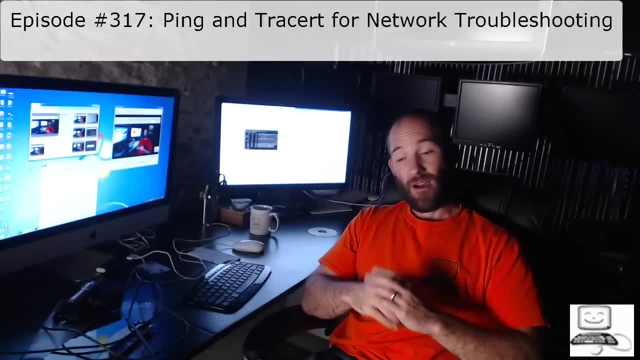 before it hit my server right. so sometimes you would see that it would get like two routers in and then fail. well, then I call them up and I tell them it's their problem. other times I could see that I got three routers in, which is, I think, how many routers my server was in, and then it failed at that point. 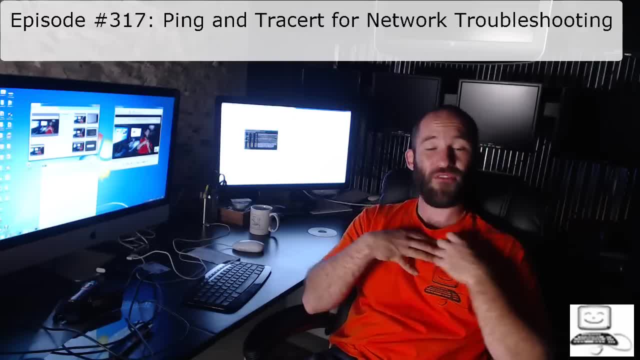 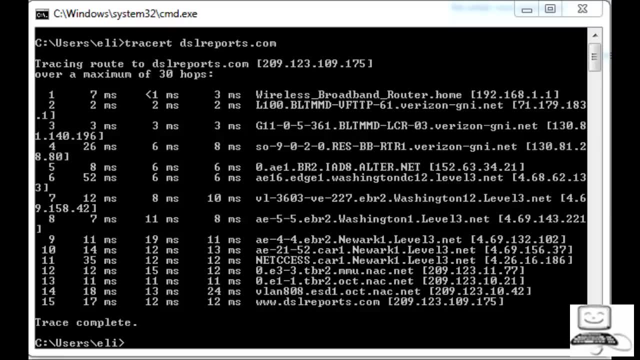 which I knew meant that it went through all their routers. it failed right, and then at that point I could see that I had my server in and then failed at my server. so that's how you can use this traceroute command. the final thing that is really, really useful in the real world is being able to tell: 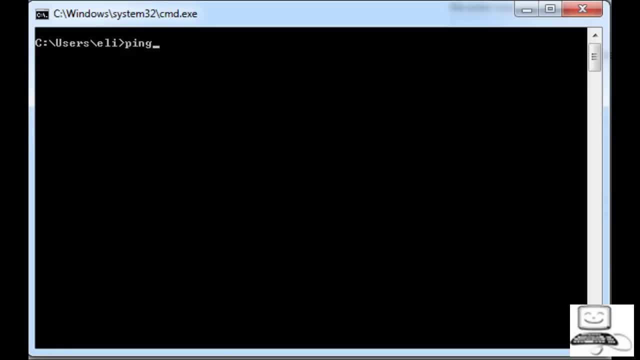 ping the number of times you want to ping a device. so I'm going to ping the computer test. so that is the computer test and I can do hyphen in and then say how many times I want to ping. so during a normal ping process in Windows it only. 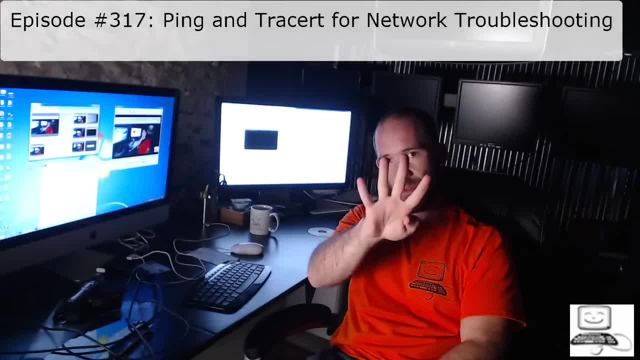 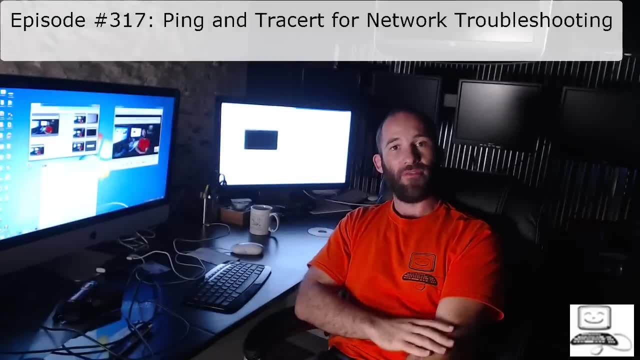 pings four times. in Linux it goes on forever, but in Windows it only pings four times. well, if I'm waiting for a server to come online or if I'm waiting for a server to go offline, using the ping command is a really easy way to. 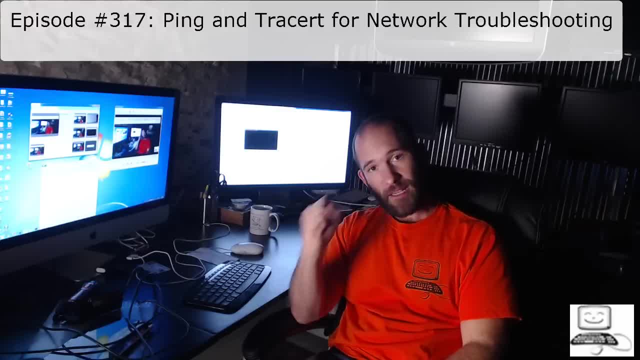 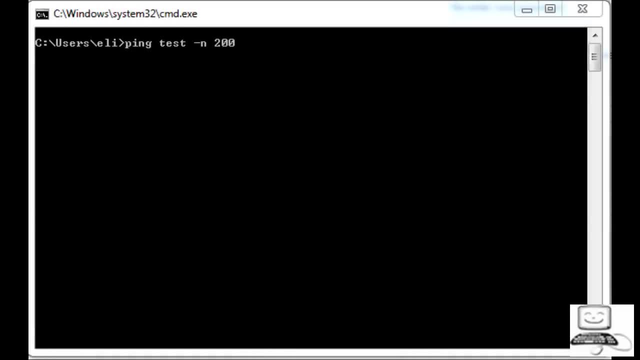 know when that has happened. I can simply just keep peeing the device until I see it come online or go offline. so with this example, what I can do is i can do ping test, hyphen and 200. so it's going to ping the computer test 200 times and 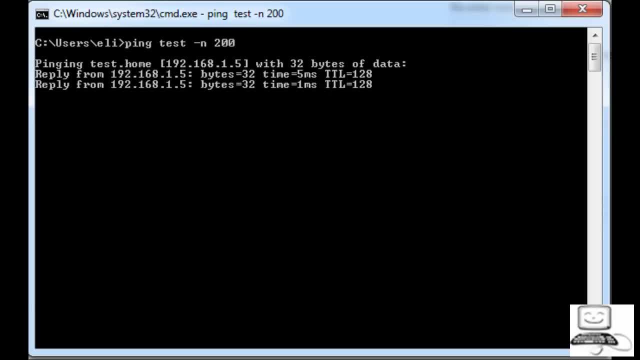 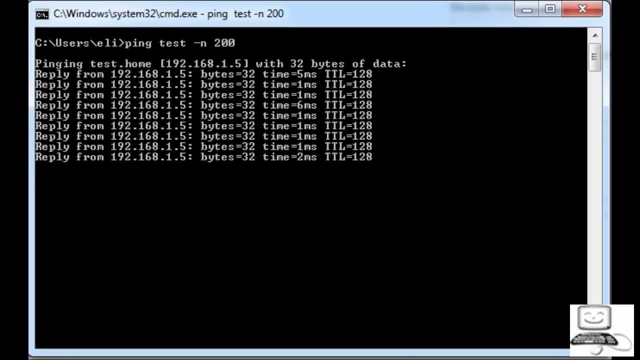 then all i have to do is i just have to hit enter and now, as you can see, it's pinging away. so test is the ip address of 192.168.1.5. and now i'm going over to the computer and i'm just being mean to it. 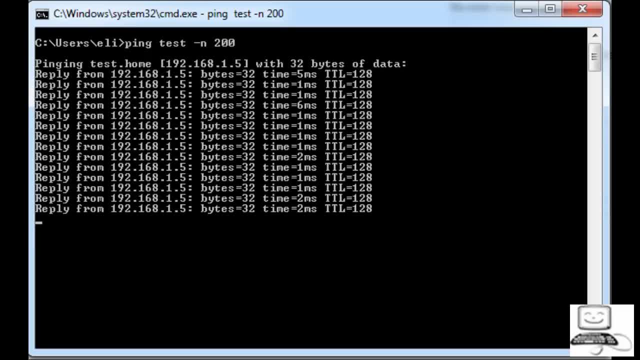 and shutting it off right now and, as we can see, right as i shut it off, it no longer applied request timed out. now request time has got to keep timing out, to keep timing out, keep timing out. so that is a very easy way to see if the computer has booted up yet or has gone down. so a lot of. 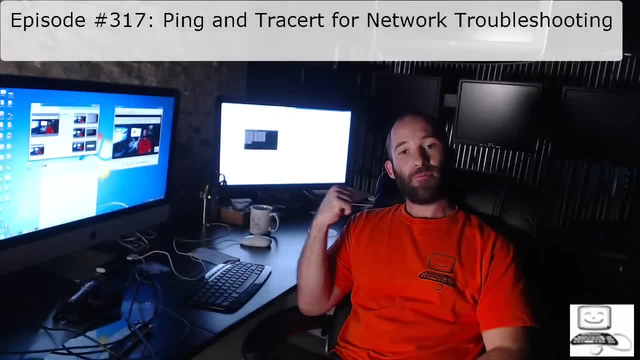 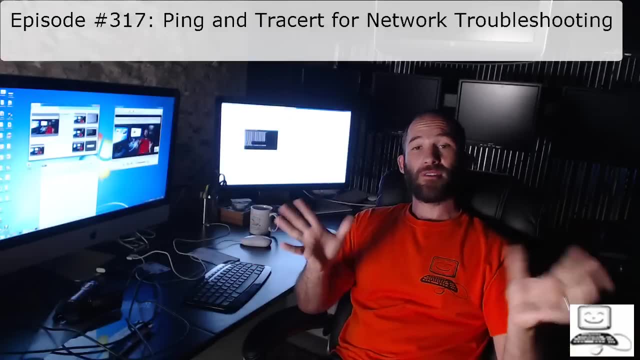 times again when i'm dealing with a lot of servers, i will run this ping command because i have to reboot a server and when you start dealing with things like small business servers, they take a long time to reboot. small business servers take like 10 to 15 minutes to reboot sometimes, and so